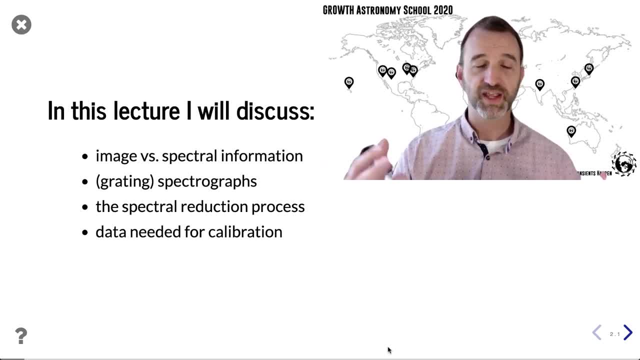 There's actually a lot of similarities between the two. They're very much the same thing, but there are some practical differences between the two, So I'm going to focus on those differences. I'm going to tell you a little bit about how we obtain spectra as astronomers. 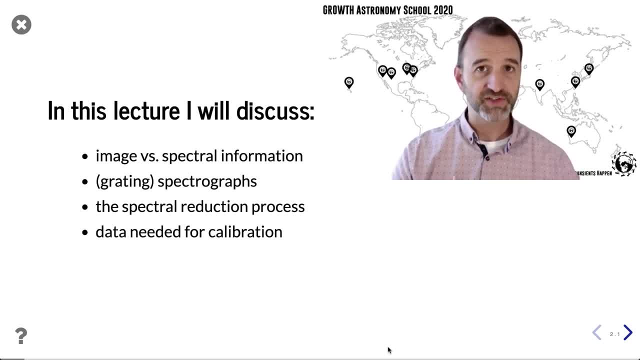 So I'm going to tell you how spectrographs work. I want to make sure you have a basic understanding of the operating principles behind spectroscopy. And then I'm going to talk about data and how we actually go through the steps of analyzing that data to remove the signal that we're interested in. 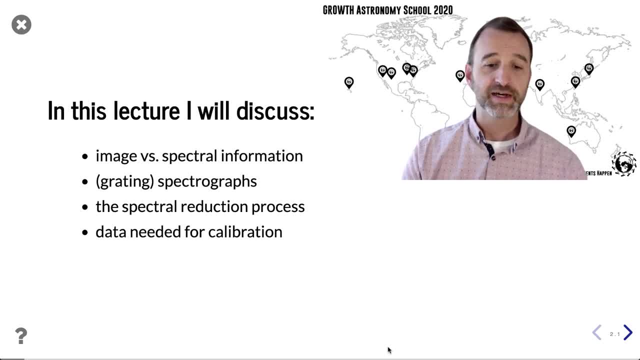 A lot of the same steps that are involved in photometry, but the big thing to keep in mind is that when you have spectroscopy, instead of just having one, you have many, many bandpasses- hundreds, maybe thousands of bandpasses, maybe more- that you're dealing with all simultaneously. 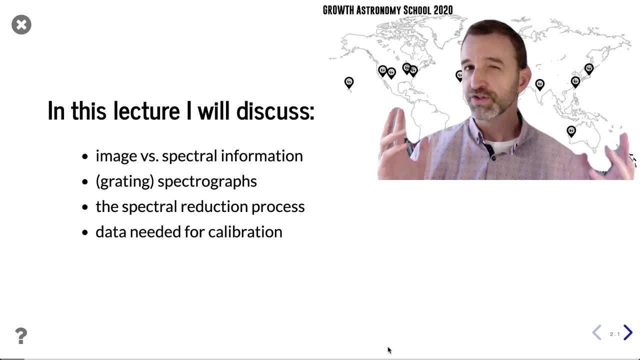 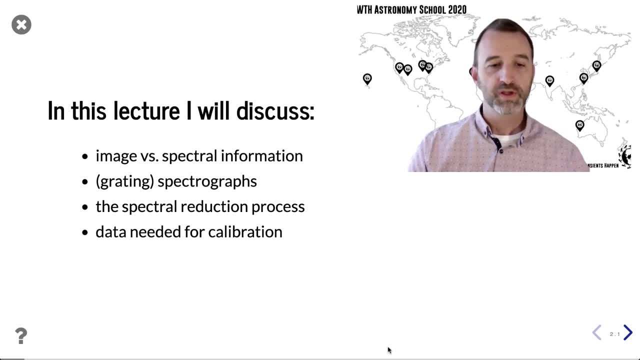 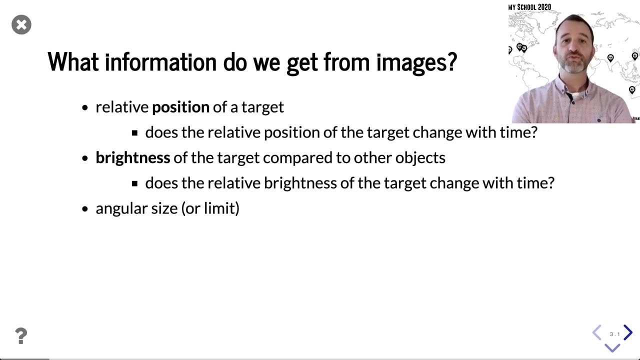 So, while it's the same steps as doing photometry on some level, you just have to have some ways of handling it all in one go. All right, so we'll first start by talking a little bit about imaging data and what we get from that. 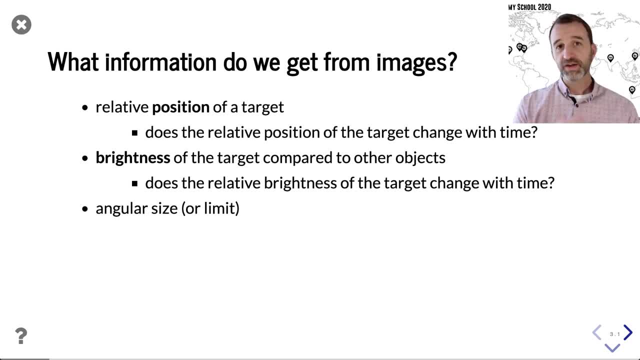 So we got a little bit of an overview of what we can compare to what we get from spectroscopy. If I give you an image of an astronomical source, you can look at that and you can say, hey, there's something there and there's not something there. 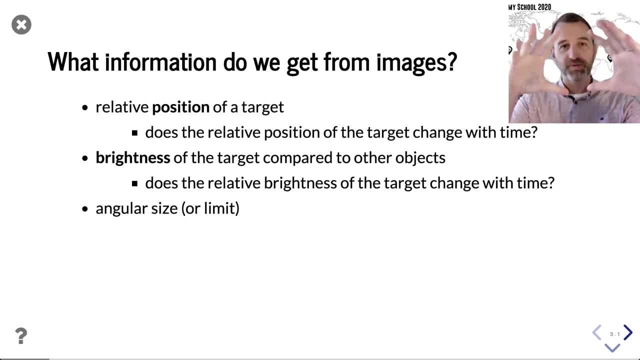 Alright, so you have some spatial information about what's inside that area of the sky And you can see the relative positions of the objects And you can say, if you take images over time, if one of those objects changes position, it tells you something about that object. It tells you it's probably pretty nearby. 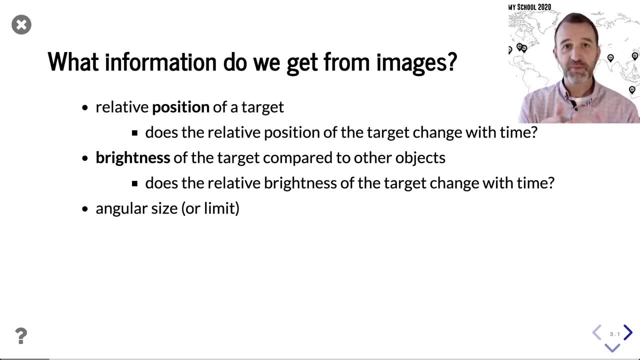 Because if it's very far away, that wouldn't, that wouldn't affect that to happen. So there's some information contained just in the position, information of targets. You can, of course, look at the image and say, hey, this thing is brighter than that thing. And again there's something, some information that's being conveyed by that. Maybe one of those objects is closer, maybe one is farther away, but you're learning something about the relative differences between those targets. 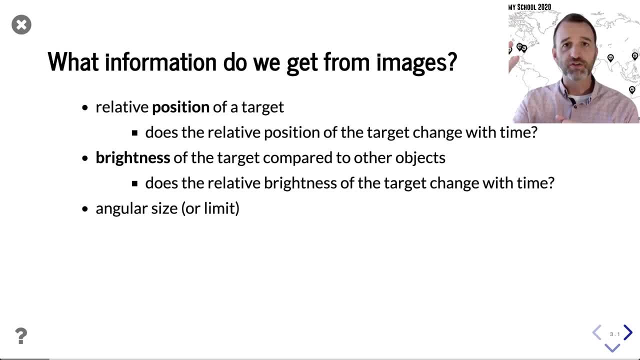 And you can look at changes over time. Maybe one of those objects is getting brighter and fainter over time. That's telling you something about the physics of that object. You can also say something about the angular size. if you haven't image, you may not know the physical size, but you can say: hey, that one. 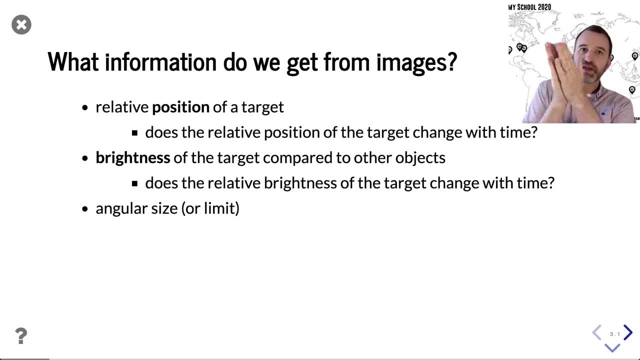 spends an angle That's this big and this one spends an angle that's that big, or maybe a target is at the below the limit of your sensitivity. So you can say, well, that one is just a point source, As far as I know, and that again tells you something about it. If you have just one object, that's very. 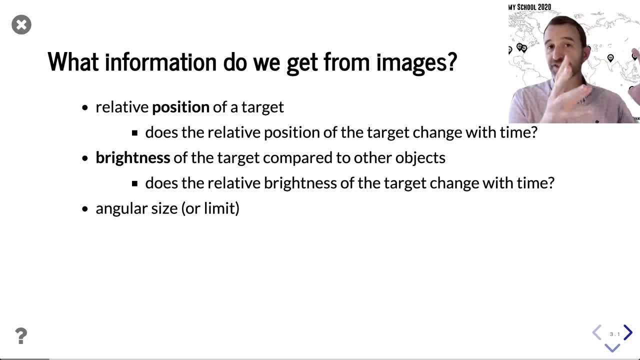 far away it's going to just look like a dot. but if you have a collection of those dots and like, say, a gallery, then that would cost you too much galaxy. then you can say, hey, we got a whole lot going on there. Of course, one of the most- 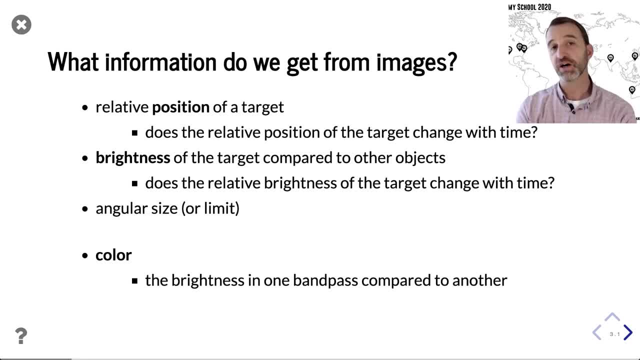 important things you can do with photometry is you can assess the color of an object. That's just the relative brightness in one bandpass compared to the other. That's telling you something again about the physics of the object, If it's a bluer object or if it's a redder object. maybe that's. 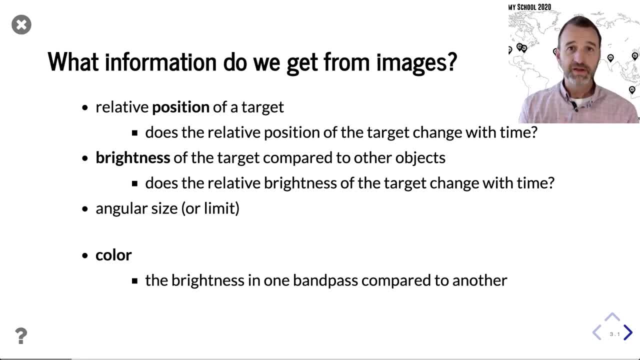 telling you something about temperature, or maybe it's telling you something about dust. There's some information that's contained in the color. Obviously, the more color information you get- if you get different bandpasses- you can get a better picture of what's causing those color. 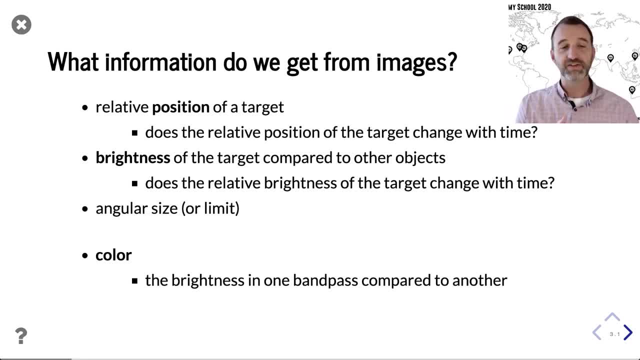 differences between one object and another. That is actually what leads us into spectroscopy We're just going from. instead of just having one black and white image to we have two images and different bandpasses to. we have many, many, many, many, many, many, many different bandpasses. 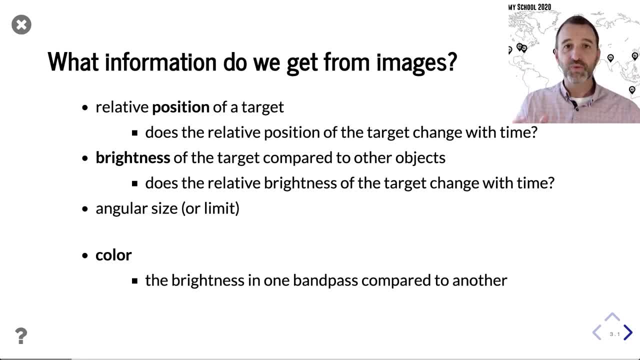 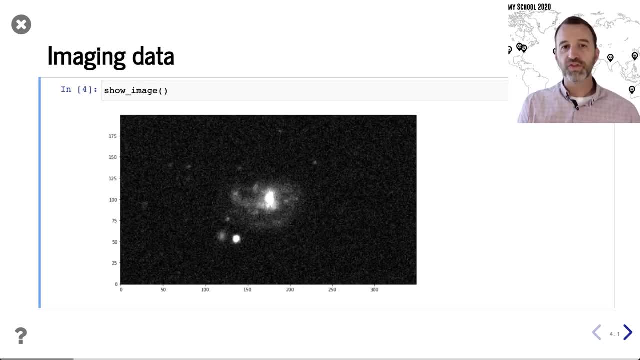 all with different flux densities. We can use that information to learn something different. Let's start here with an image. This is a real image that was taken by Sloan Digital Sky Survey. You can look at that image right away and you can say something about that object. 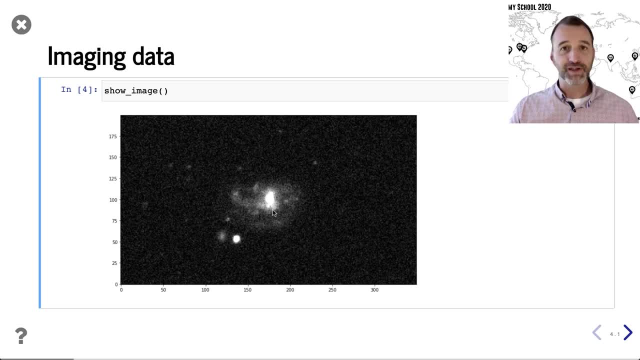 This object that we see on the screen here is probably a galaxy. I can say that because it's extended. The mission is not just at a point source. Even though it's very far away, we can see the light spread out in our imager, Whereas this source right here that could be a star. 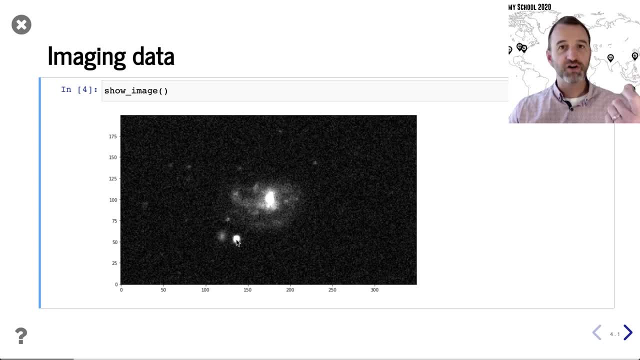 could be a supernova related to this, but we can't resolve that object. There's maybe a little galaxy here, So there's a lot of information you can see just by looking at this, But you can't tell me much more than that. You can't tell me what this galaxy is made of. You can't tell me is this: 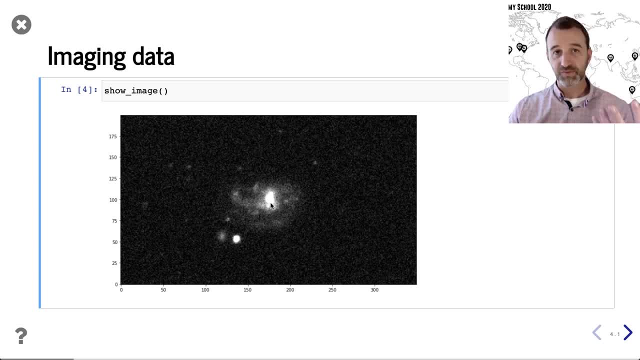 galaxy moving towards us or away from us. To do that, that's where we need spectroscopy. So Sloan Digital Sky Survey actually took a spectrum of this galaxy as well. So they put a little aperture around this core of this galaxy and they pass it through a spectrograph- the light they pass through a spectrograph. 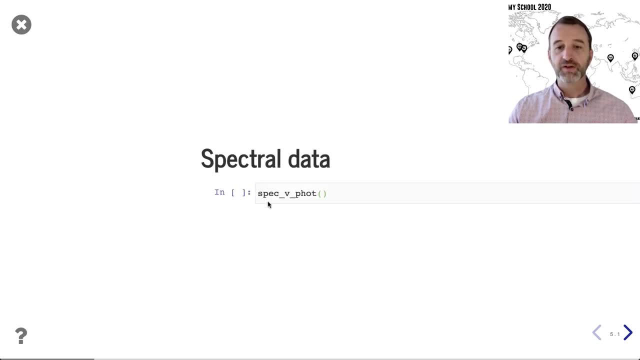 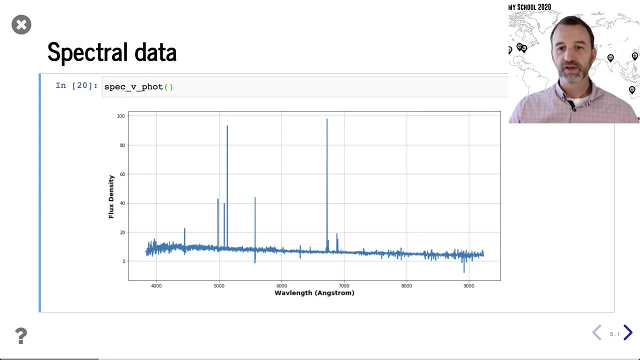 and they learn something about this object. So let's take a look at those data. Let's start with just a spectra Twice. And this is the spectrum from the Sloan Digital Sky Survey. So you can see we have wavelength here in angstroms, And this is thousands of different bandpasses here. 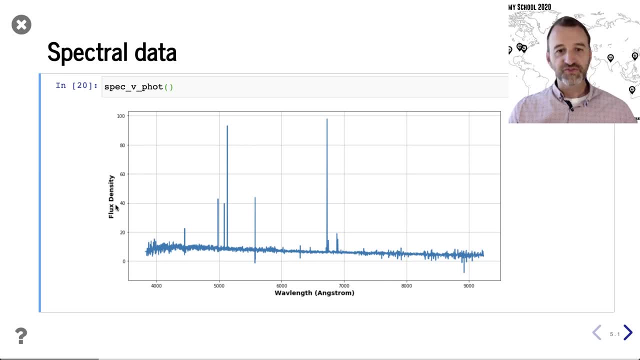 Right, thousands of different little bins that I'm plotting here, And this is flux density here, And you'll notice that. okay, first there's this continuum, So basically any wavelength you pick, you're getting some light And it's pretty smoothly connected here. But on top of that there's these emission lines that pop up. 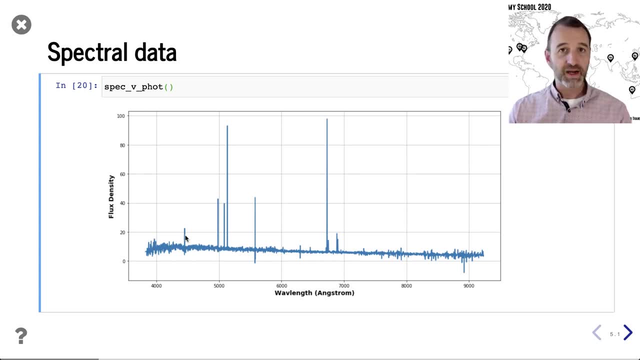 And these emission lines are telling us something about that object. It's telling us it has gas. We're learning something about the chemistry just by looking at the spectrum here. We can also tell that there's starlight in here. So there's gas in the galaxy and there's starlight. 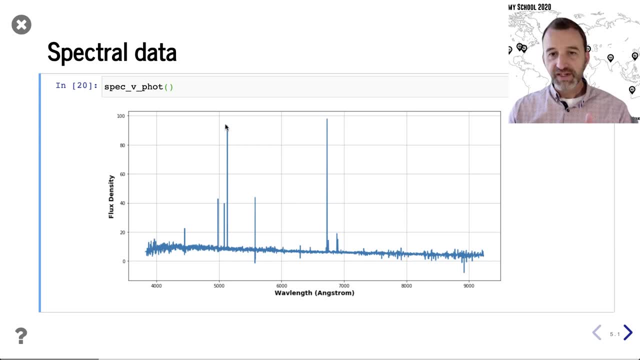 So all this information is contained in here And if we look at these and we can either find- hey, I know these lines, they're oxygen, because in a laboratory I can make a spectrum that looks a lot like that, except for it's shifted a little bit, now we can actually figure out what. 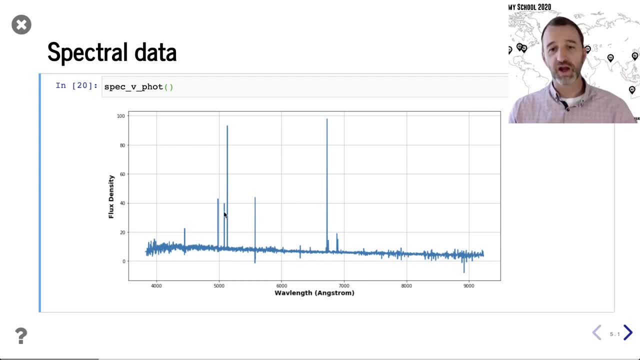 the red shift of this galaxy is. We can say: how fast is that galaxy moving away from this? So all that is contained in this spectrum. So let's compare now what we're getting from spectroscopy to what we were actually seeing before in photometry. So what we're doing with photometry. 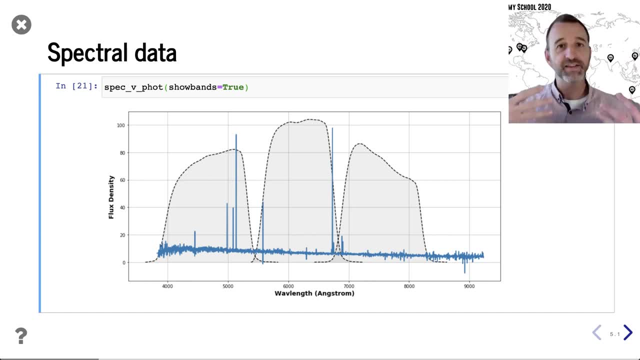 is we're taking the same light that we're getting from that galaxy and we're just using bigger bins to image it. So that image I showed before I think is with G-band here. So we have a band that spans 1,500 angstroms. 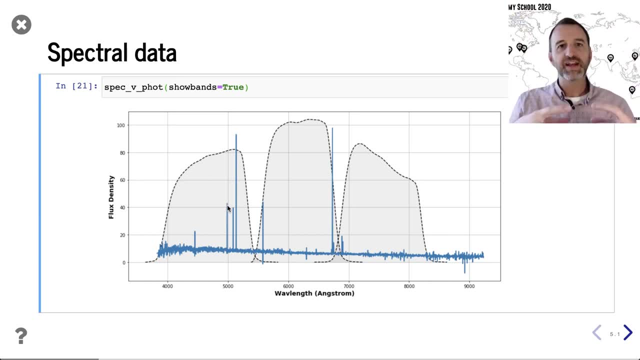 and any light that we get within that spectral bin. we're all integrating together. So we're integrating, we're kind of doing a convolution of this filter function here with this spectrum here, And from that convolution we get one number: 15.6.. 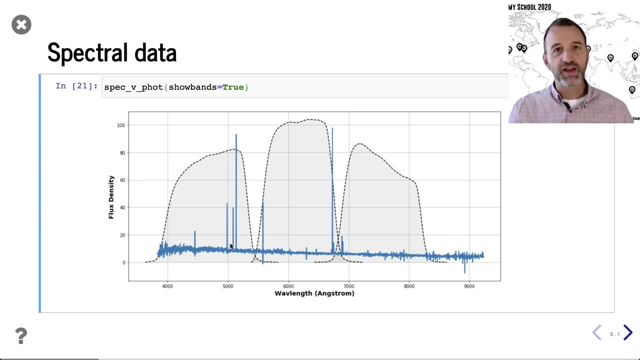 Now that's the number you get for all this right here, For all these thousands of little different spectral bands that we get in the spectrum. you only get one number. So you can see, if we just had the photometry here, we can't directly say: 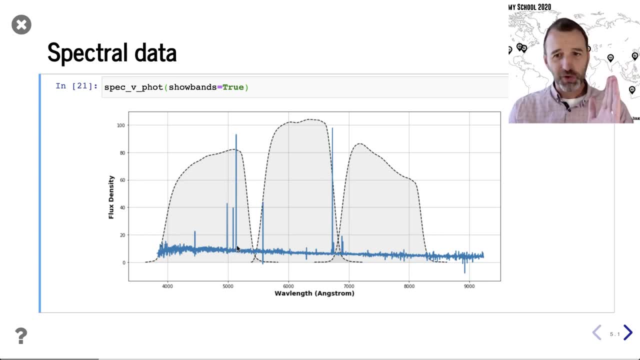 oh, that object has oxygen in it. We might be able to guess, but we don't know for sure. And we might be able to guess at the redshift, looking at how the light falls off with color, but with spectroscopy you can get a very precise measurement of it. 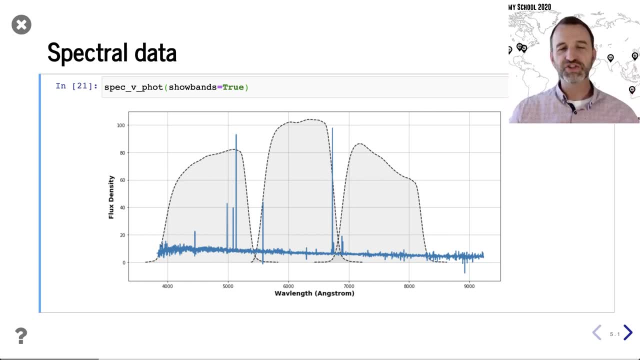 So, again, all the difference between spectra and imaging is really not so great. It's just that your band passes are smaller. So instead of having huge band passes that span thousands of angstroms, maybe they only span one angstrom or 10 angstroms. 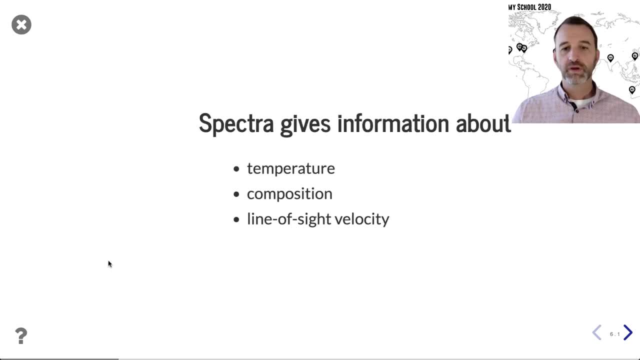 They're much, much smaller. So through the spectra you can evaluate what the temperature of an object is. You can look at the composition, as I've been saying, the oxygen or hydrogen, silicon, sulfur, what's in it, And you can also do this line of sight velocity. 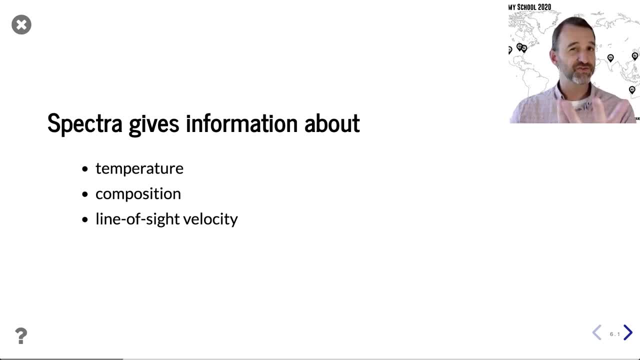 So there's a lot of information that you can pretty directly get from spectra that it's very hard to get from broadband photometry, Of course, if you take your photometry instead of doing those broadbands, if you did more narrow bands and you did more of them. 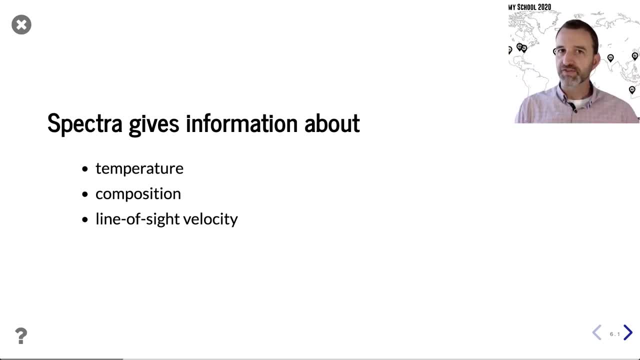 then you'd get actually a better picture of what that galaxy was made of and what its temperature and maybe even redshift were. But what you're doing there, and really what you're doing with photometry- broadband photometry- is actually low-resolution spectroscopy. 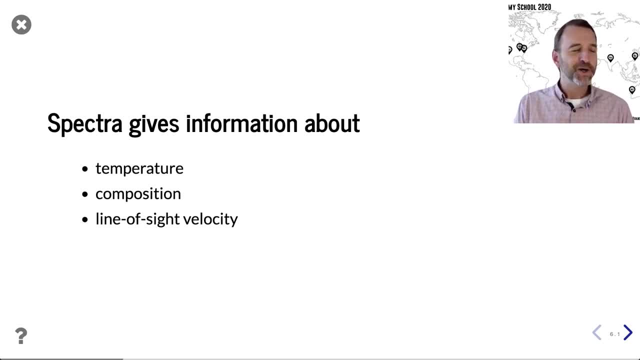 You're just doing it in sort of in an inefficient way. If you wanted to know what the spectral energy distribution of an object is, you can take one image and take another image and take another image, each in a different narrow band, or you can get one spectrum. 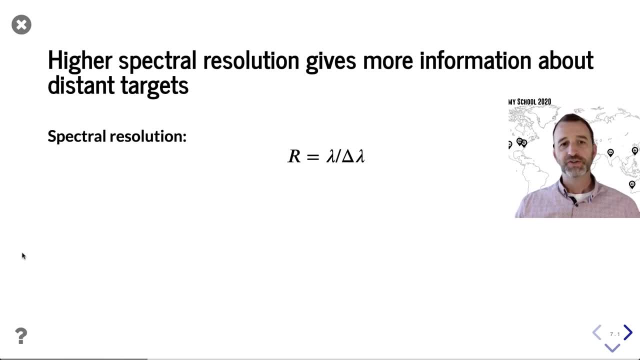 where you get all that information in one go. So the key difference really between what we call photometry and what we call spectroscopy really just has to do with this quotient, this quantity here, resolution, spectral resolution, which is just a ratio. 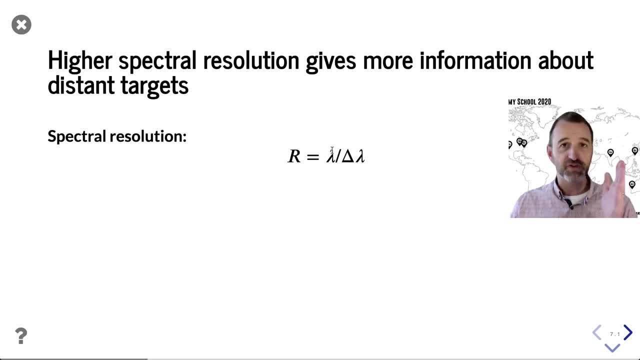 of the light wavelength of the light that you're looking at to the spectral bandpass. So delta lambda here is telling you how wide your bin is in angstroms and lambda is telling you what the center wavelength of that bin is. So for photometry, 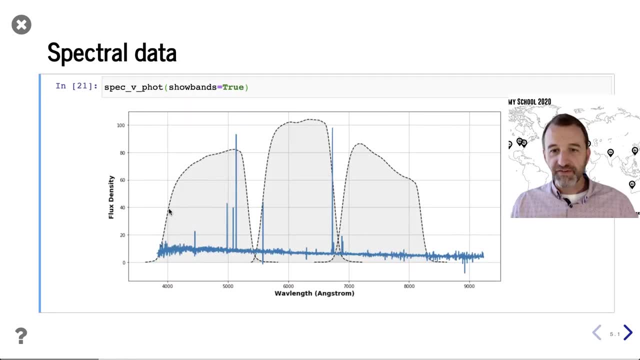 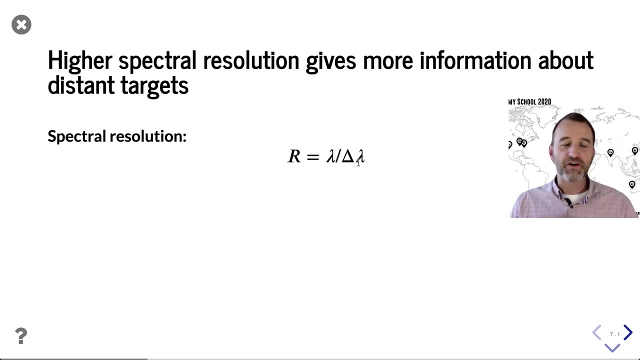 we have bandpasses that have a delta lambda of 1,000 or so and they have a lambda of around 5,000.. So you have a resolution of 5,000 divided by 1,000, so about five. 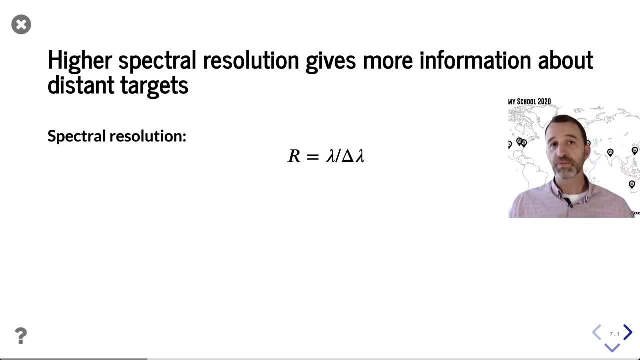 So broadband imaging, you get a resolution of five, Whereas with spectroscopy, typically, you're working with resolutions of 1,000 or could be even higher. You can go up to 100,000.. So there's an old adage that a picture is worth 1,000 words. 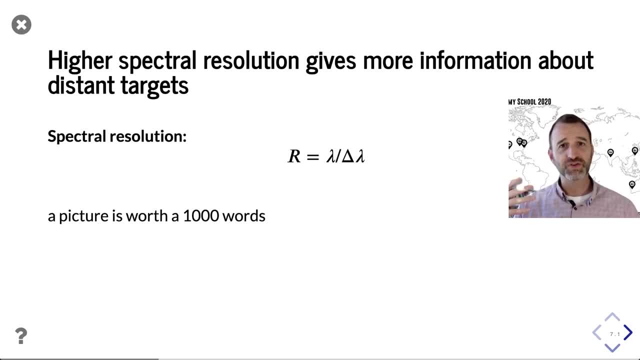 So if you work out the math here, instead of doing a resolution of five, if you're doing a resolution of 500, you get 100 times more information. So spectrum must be worth 10,000 words. It's just math, people. 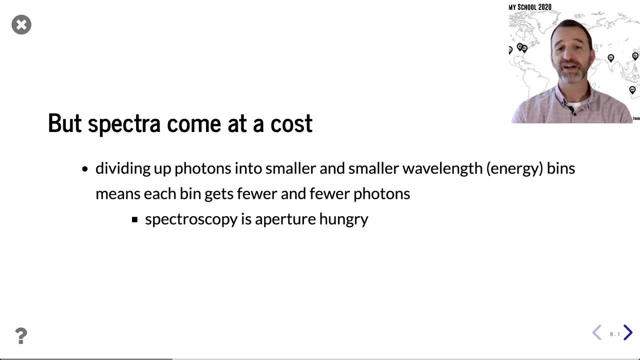 But there's a cost for those words. Spectra are difficult to get because when you take all the light that you're getting- and these are- you know if this is a faint object, it's far away, you're not getting so many photons here. 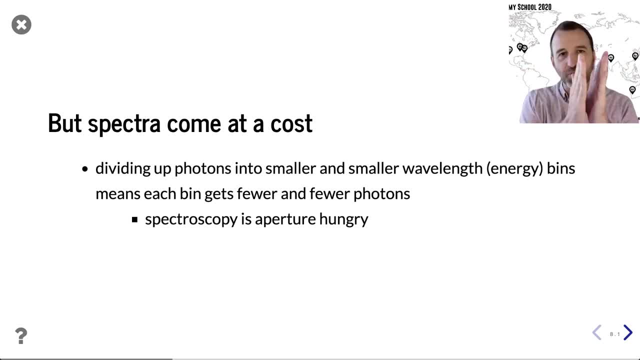 And when you start spreading out that spectrum and just dividing it into smaller and smaller spectral bins, each one of those spectral bins is gonna get fewer and fewer photons in it, So it becomes hard to get a significant detection in each one of those spectral bins. 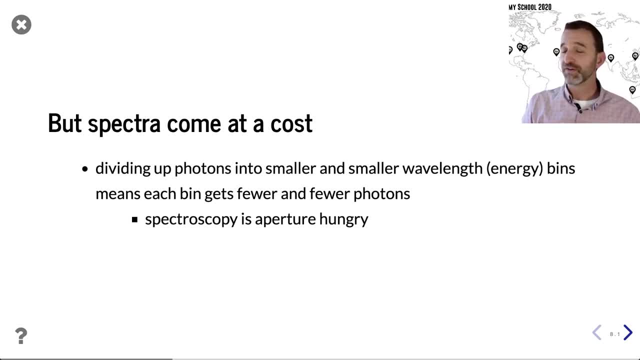 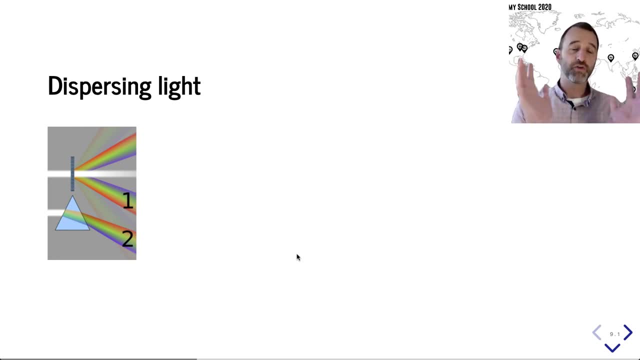 So what you really need when you start doing spectroscopy: if you wanna do spectroscopy of faint objects, you really need a large aperture telescope. Okay, so hopefully we've been motivated now why we want spectroscopy. You know it's in one shot. 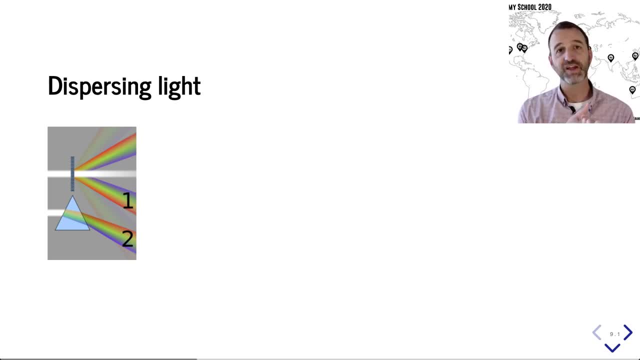 You can say what the composition is. temperature, radial velocity is of a target. That's great. How do we go about doing that? So now let's talk a little bit about how we can make a spectrum. You probably already know this. 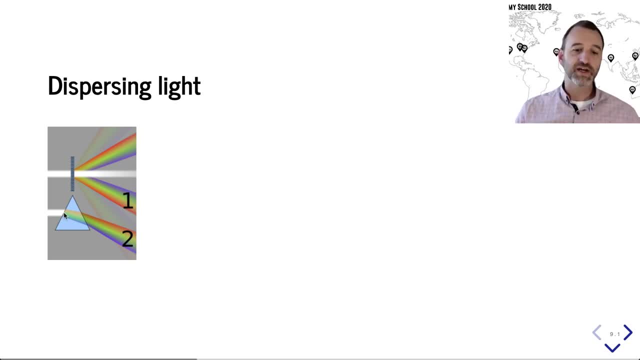 You know that you can take in light and that light travels at different speeds for different mediums, So depending on wavelength. So if you're very clever about this, about how you organize your media, you know going from air to going to glass, to going to air again, 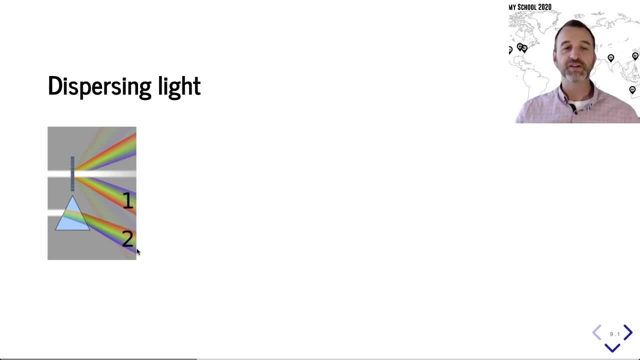 you can make a prism and that will take white light and disperse it into a spectrum. This is sometimes used in astronomy. As professional astronomers, we sometimes deploy prisms, but actually we don't use these too often. A more common is something like this: 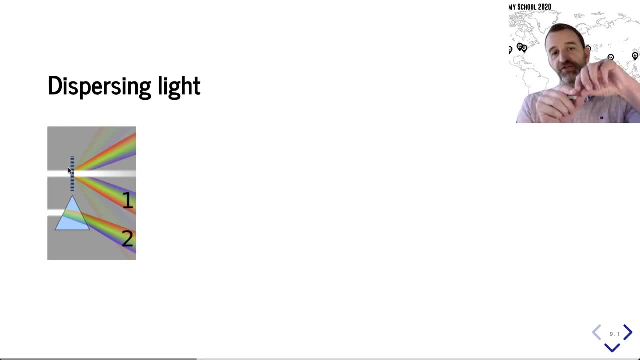 This is a grading now. So in a grading you have some material which has a bunch of a pattern in it. Let's start with just a bunch of slits in it. Bunch of little notches cut through it so light can pass through those slits. 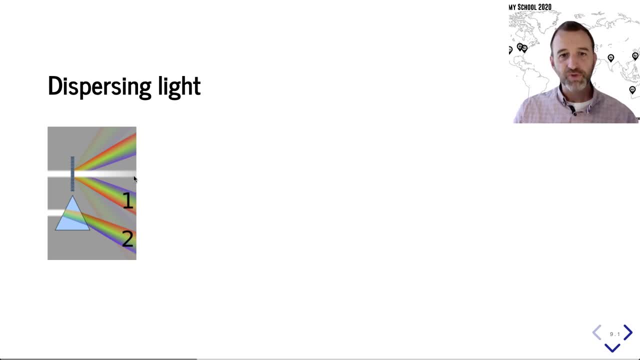 So what happens is some of the light goes straight through and you get an image, But at angles, when you move away from there, you also get light that's going in that direction. And if you get light going through one of those slits, 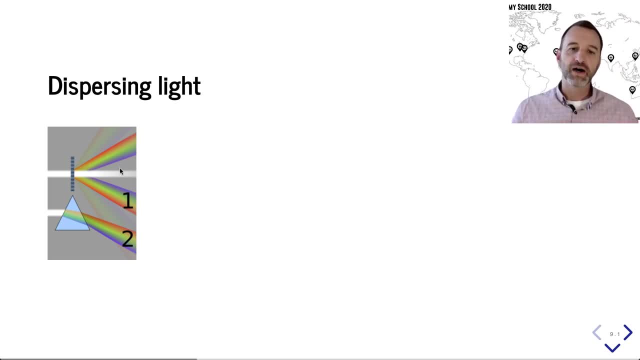 and another of those slits. they come together, they can form a bright spot. that's wavelength, dependent on your detector. So instead of just getting one image, you actually get an image and then you can get a spectrum and you get another spectrum that mirrors that. 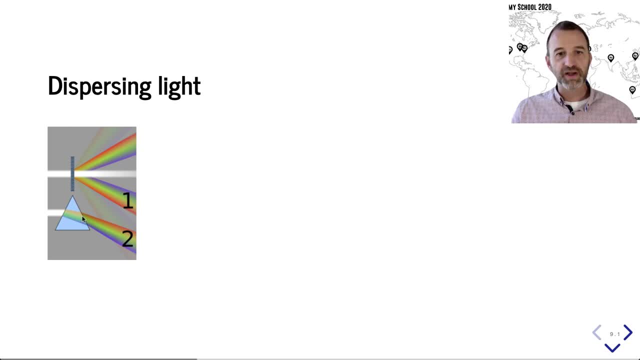 This is all symmetric And you actually get these higher orders of spectra coming up as well. How does this all happen? Well, you guys have probably done this experiment before, where you take a laser and you have a double slit. you shine the light of the laser through. 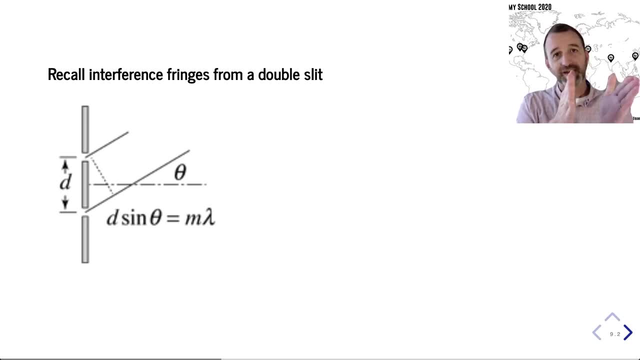 and, depending on the path length difference, you're either going to get constructive or destructive interference on some target screen. So let's just work through the geometry on this before You have some slits in some mask. These are separated by some distance. 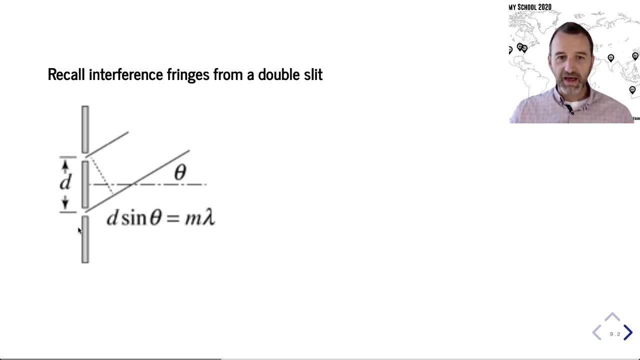 And what you care about is when these two paths reach your detector off at some distance, are the wavelengths going to be in phase, And you can figure that out by looking at the path length difference here. This is d sine, theta here, or theta is this angle away. 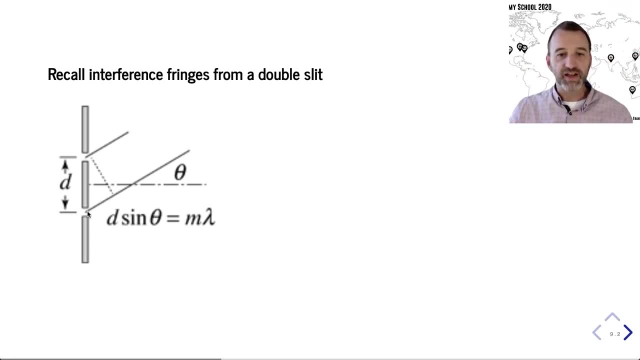 from the direct line of sight here, And if this quantity is an integer multiple of the wavelength that you're using, so you got that laser at some wavelength. if it's an integer number, that means that light's coming in for one slit and light's coming in from the other slit. 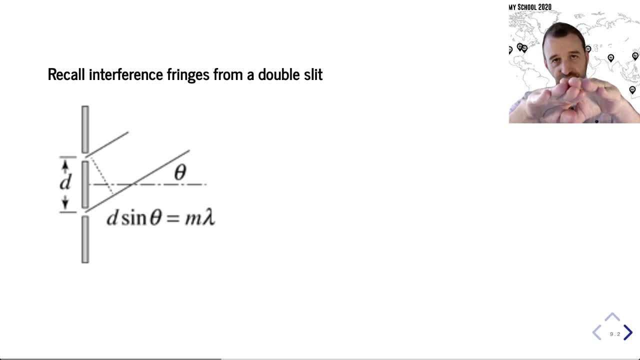 and they're going to come together in phase at your detector, And so you get constructive interference. If it's a half integers, it's not an integer, then you get destructive interference. You got a wave that's coming up, wave that's coming down. 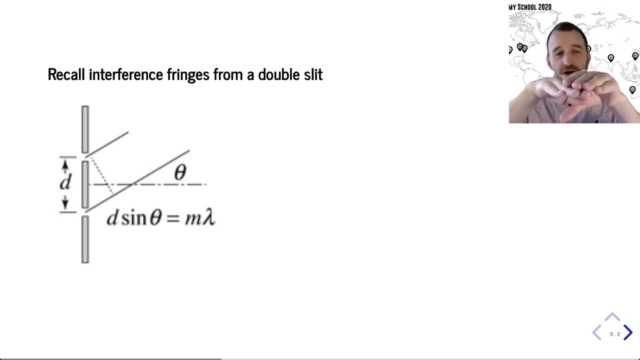 you're going to get destructive interference, And so they won't. they'll destructively interfere, which of course means that that's not going to happen. You're not going to get those two photons going in that direction. They're either going to be absorbed or scattered. 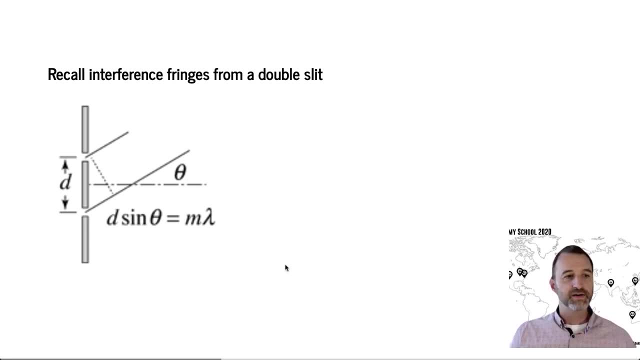 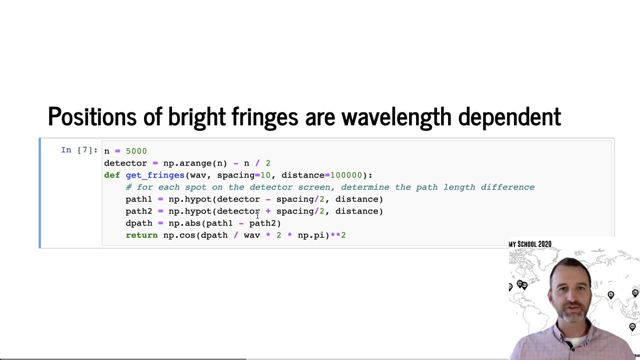 but they're not going to go to your detector. All right, so let's just do a little kind of toy demonstration of this process. You've done this before, but there's an important wavelength dependence that you may not have considered before. I want to make sure this is clear to you. 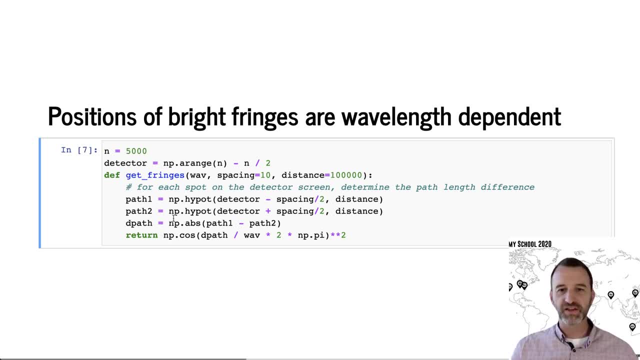 So I've got a little fake detector here which is pretending there's a screen and there's two path lengths of from two different slits in there And we're going to look at whether we're getting constructive or deconstructive interference. 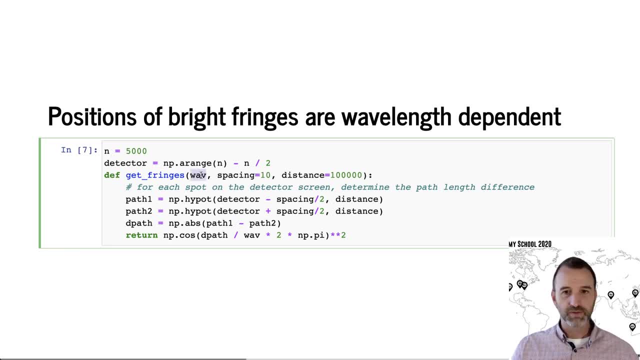 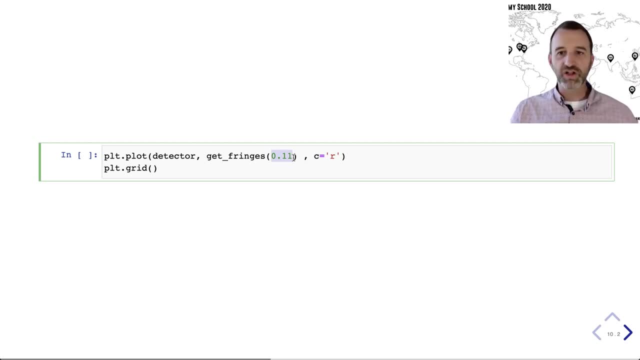 depending on what the wavelength is that we're supplying. So first let's consider some wavelength of light, So 0.11 in whatever units. maybe this is some red laser that you're shining through the slit, And when we do that, this is what you're getting. 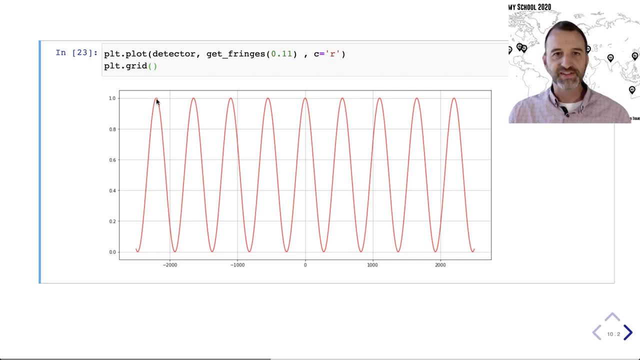 So this is just intensity plot here. So you know: intensity one, you got constructive interference. intensity of zero got destructive interference. So on your detector there's some center line here at zero and the two waves are in phase and they come together. 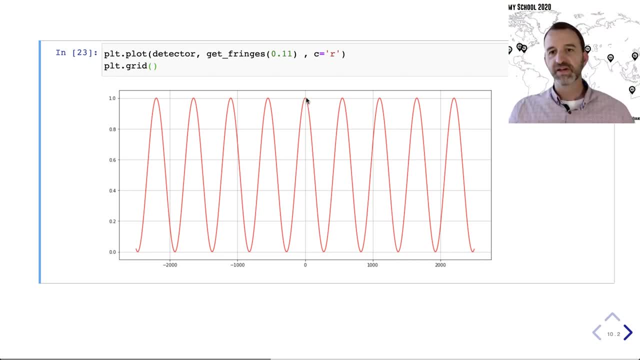 and they make a bright spot there And then, when you move away from that, you get destructive interference. and then you get constructive and destructive- constructive, destructive. So you get these bright spots as you move away, but they're discrete points. You get a point here and you get a point here. 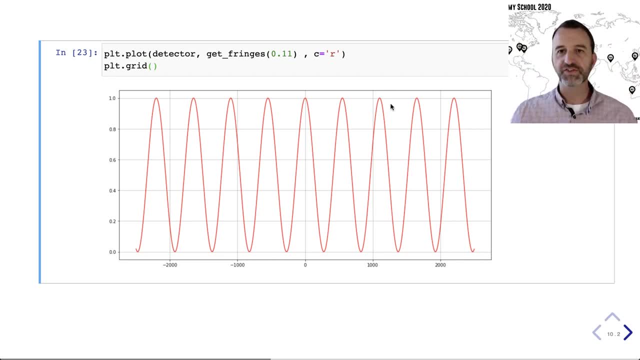 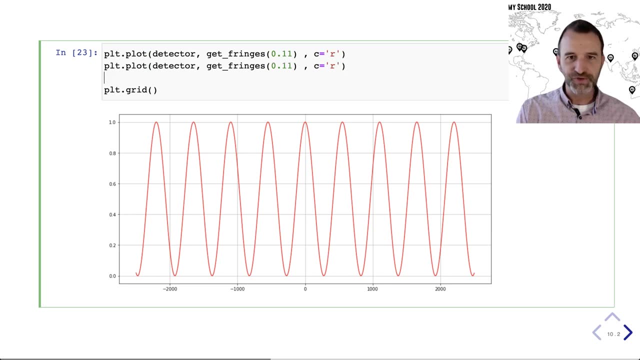 and you get a point here right. So you've all done this, hopefully with a laser, at some point. What you may not have done is use two lasers, And it's kind of a shame that we don't do this. experiments with two lasers. 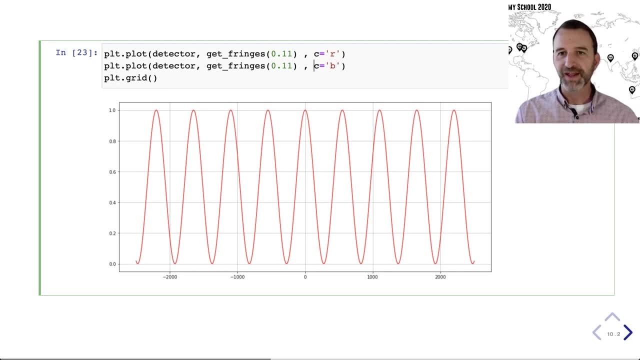 It's maybe a little more than young students can handle when we first encountered this, but let's say we had a blue laser, not just a red laser and a blue laser, but we had not just a red laser, but two lasers, red and a blue. 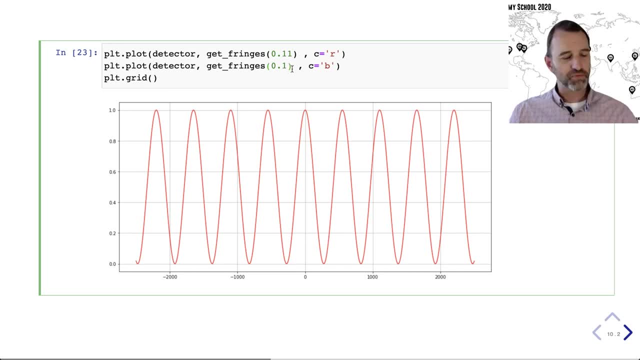 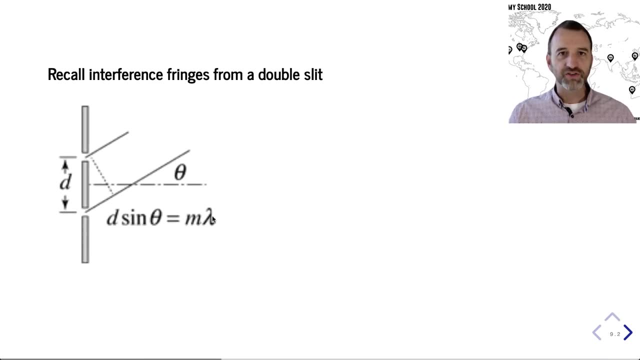 So we have a shorter wavelength here and we're gonna go through the same process And we're gonna keep in mind that there's a wavelength dependence here on where we get those fringes. So at different angles, if we have a different wavelength. 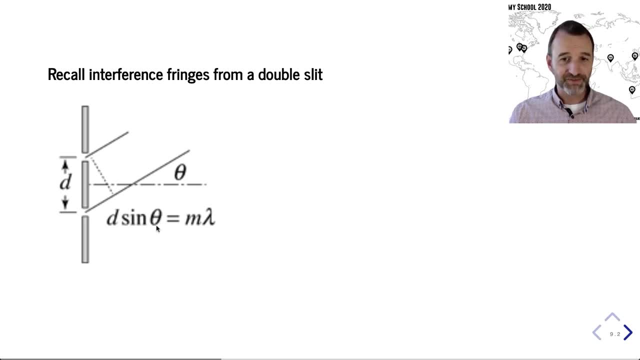 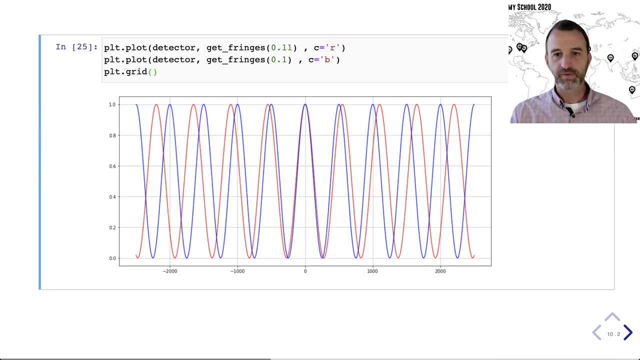 the interference is gonna be constructive or deconstructive at different angles. So that means when we go here and we add our second laser to this mix, this is what we get. So again at that zeroth order, they both come in in phase. 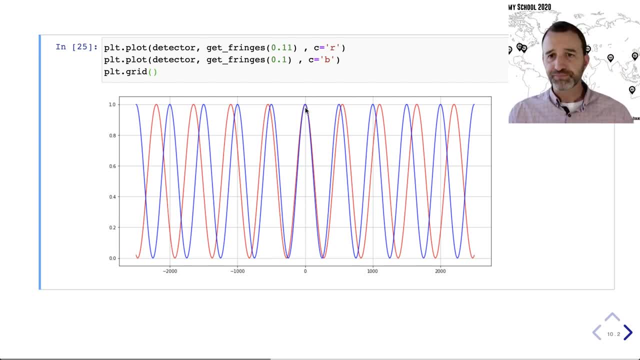 and we get constructive interference and we get a bright spot. But as we move away, we get these little bright spots moving away at different orders but at different places for different wavelengths. The red: that's our longer wavelength. You have to have a greater angle away from the center line. 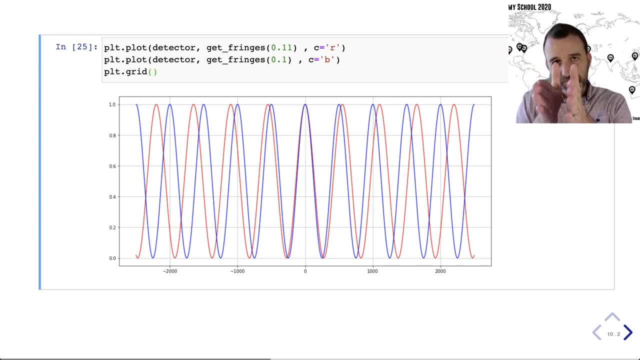 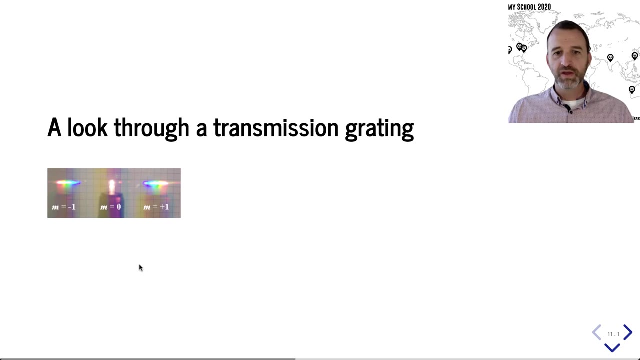 to make a bright spot at each order, The blue ones needs a smaller angle. So what we start getting here is dispersion. The light is dispersing as a function of wavelength, And this is the key behind spectraps. So this is an excellent image here, looking through a grating 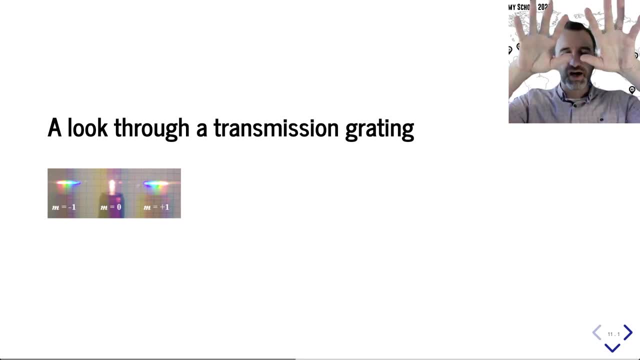 So we have in front of the camera. there is a grating which has very, very a lot of these little tiny slits in it. There's so many and they're so close together that you can't see it here. 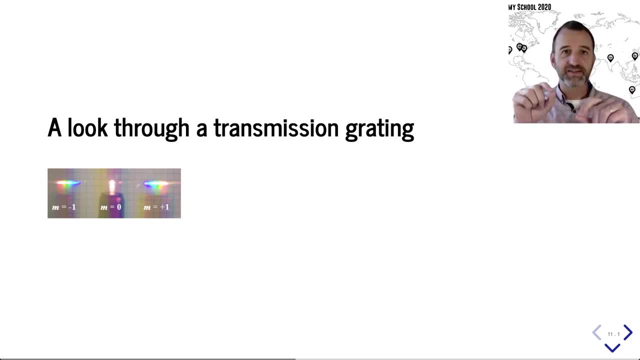 but they're all there. The advantage of having lots of slits is that you know you get a lot more light that you can pass through, but they all still have to go through slits And that means you still get this interference effect. 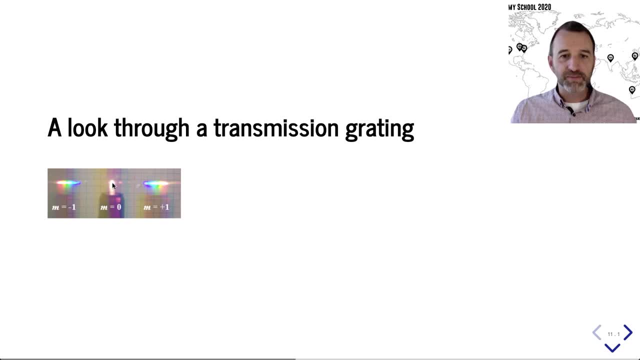 So behind the grating there's a little light bulb, here some incandescent bulb, and because of the grating in front of the camera, light is dispersed. So we get the zeroth order image here. we get the plus one order here. 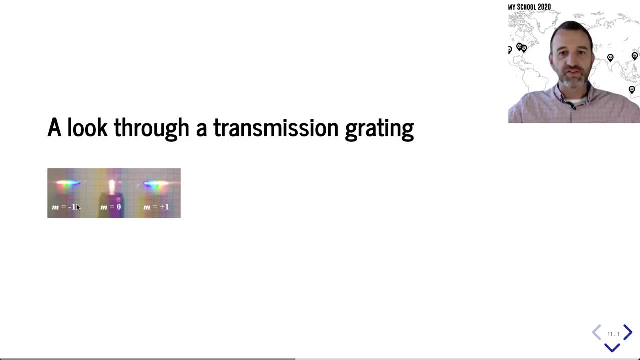 and the minus one order here. And then, of course, there's higher orders, if we could see them: second order, third order, And always note that the blue light is at the smallest angle from the zeroth order and the red light. 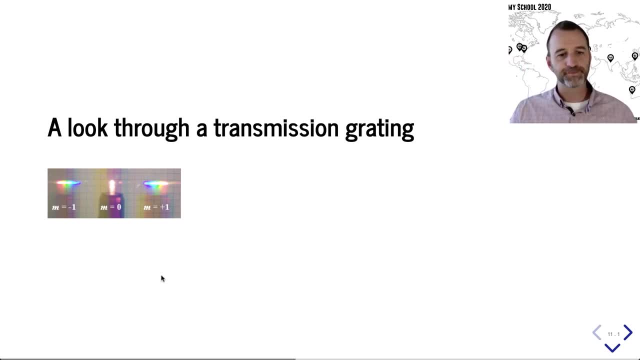 the longer wavelength is at a greater, and this is symmetric, So that's a transmission grating. We don't have to do it this way. Actually, any repeated pattern, whether light is shining through it or reflecting off of it, will cause the same effect. 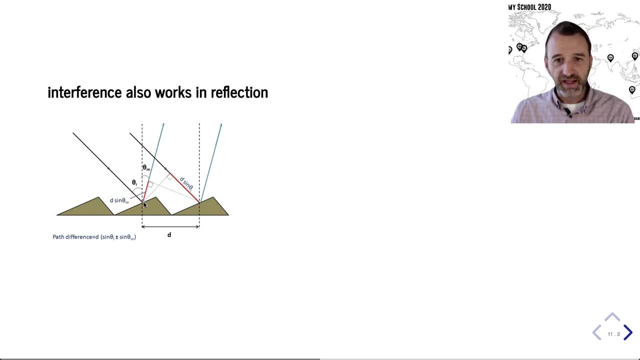 So the geometry is basically the same. You have rays that are coming in. they're bouncing off of different structures. If you have this repeated grid here, what you'll get is reflected rays and there'll be a path length difference. Again same thing. 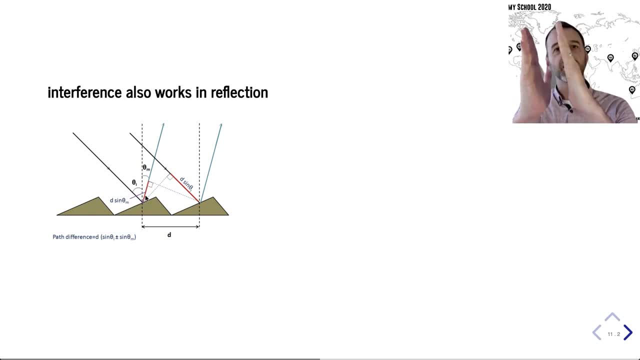 D sine theta for that path length difference. So, depending on what the angle is away, you're going to get constructive or deconstructive interference as a function of wavelength. I should note that you right now, I'm convinced that you have access- 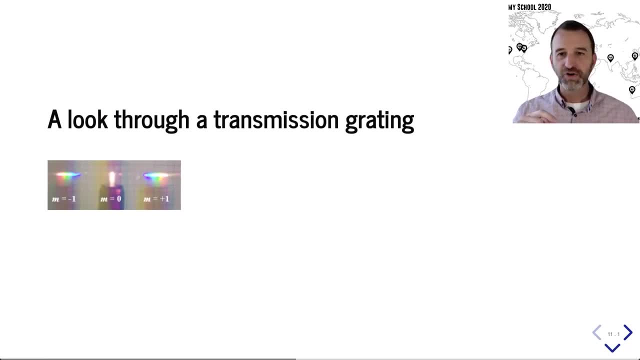 to a reflection grating just like this. Most people don't have transmission gratings lying around, but almost everybody these days, especially you, the viewer, I know you have a reflection grating at hand. It's the monitor in front of you. 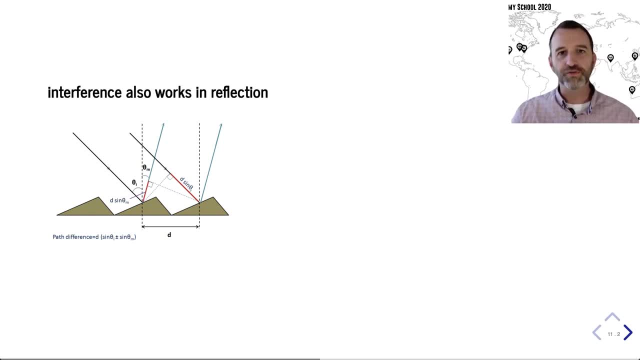 Whatever you're looking at, if you have a screen, if you're looking at this on your phone or if you're looking on a computer, that screen has a set of pixels, which is a regular grid right, And so if you look at reflected light off of that, 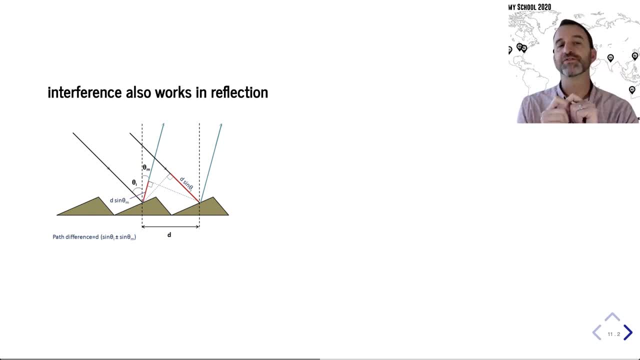 usually you're looking at emitted light, but if you're looking at reflected light off of that structure, you'll actually see spectra. So you can do this. The easiest way is if you have a phone, turn on your light. You need a point source of light. 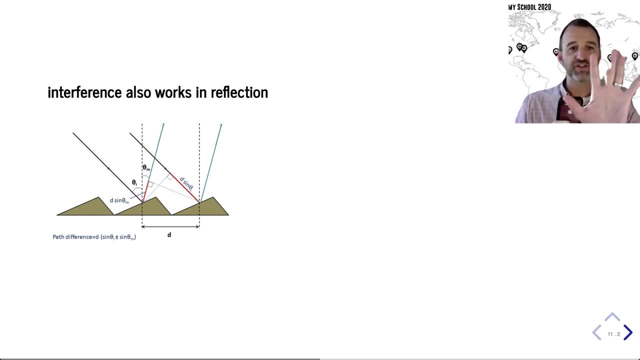 a very small, so the lights on phones are actually pretty good. And then what you look at is: you look at your screen. hold the phone like this and look at the reflection of that light in your screen, And what you'll see. 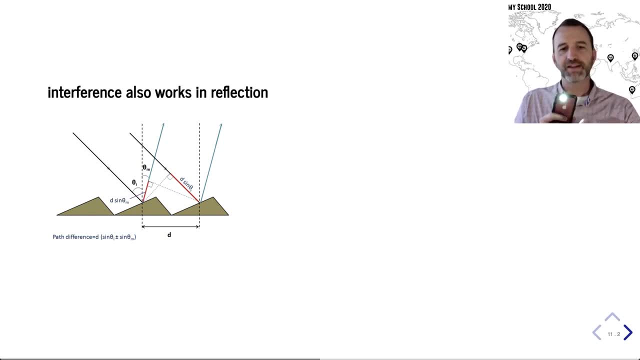 don't look at my phone, you gotta look at your phone. get your own phone and look at the screen and you'll see little rainbows coming around- the zeroth order image of the light there. All right, Okay, So that's the setup now. 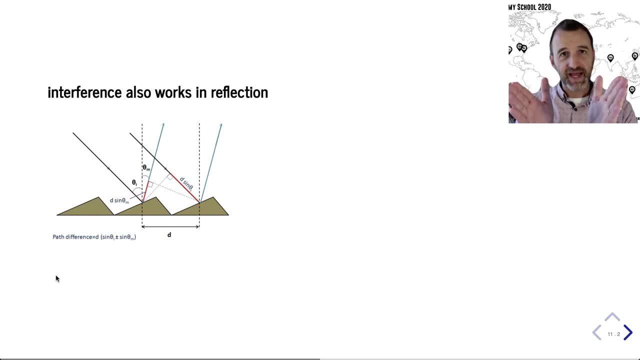 Now we know how we can make spectra. All we have to do is we have to disperse that light and then just take a picture of it And we can analyze that, just like we analyze imaging data. So let's start off now with how we actually set up. 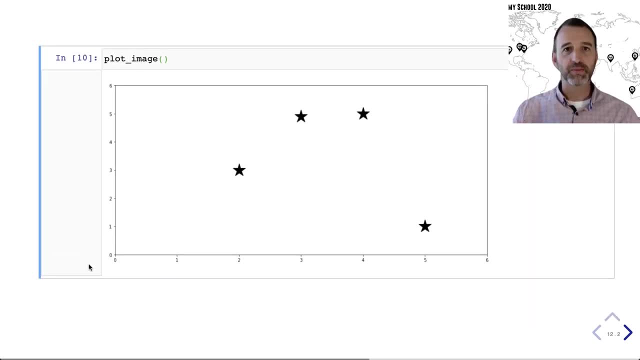 our instruments to take this data. So we'll start with just a basic image. So we have a telescope, we got light coming through, we have focus it, we can take an image. Maybe this whole thing is our detector here and we got these different stars that we can image. 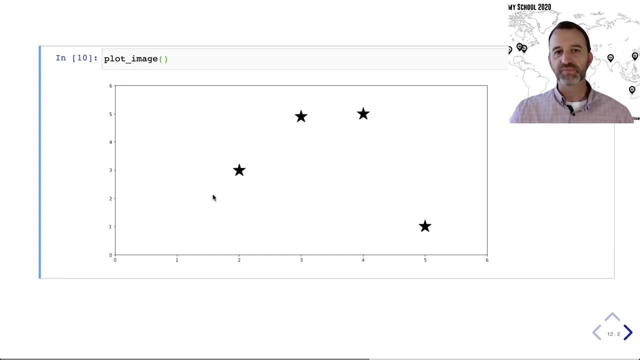 This may be right: ascensions, maybe declination. This is what we've done before. Now what we want to do is we want to disperse that light. So, somewhere in the path we're going to put in our dispersive element. 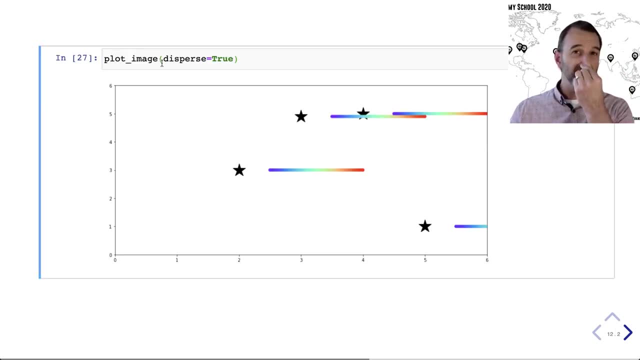 And this is what we get now. So this dispersive element could be a grism, or it could be a prism, could be a grating- I'm going to assume it's some kind of a grating. So that means you're going to get your zeroth order image. 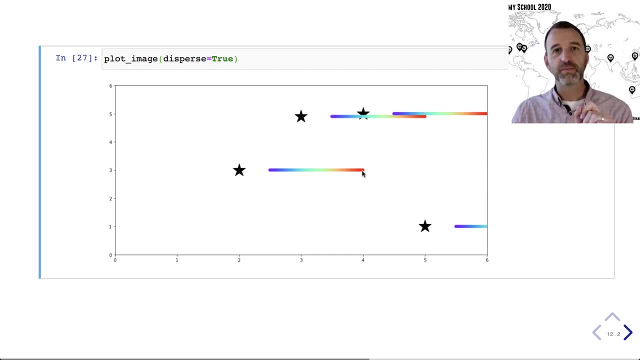 So we're still going to see stars and you're going to get some a spectra. So we're still going to see stars, Spectrum from that, And actually you probably get multiple spectrum. You get higher orders, you get negative orders. 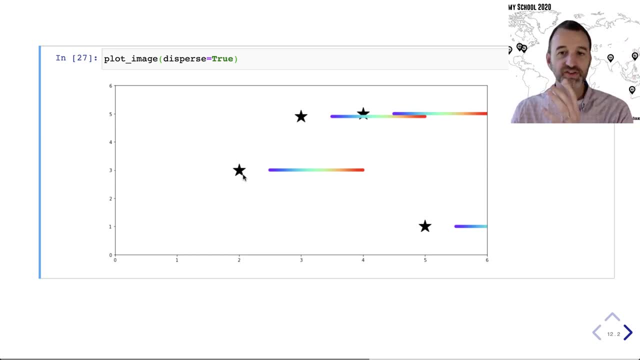 just to make it a little simpler, I'm only showing one order here, the zeroth order, in one dispersed order, So we can see what happened here. We have our dispersion axis set horizontally here, So the light is dispersing horizontally on our image. 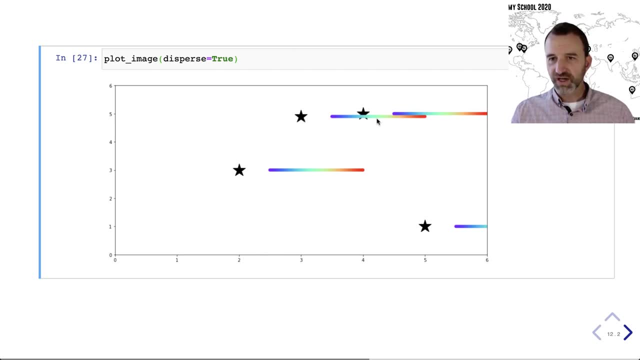 And what ends up happening now is that some of these objects were kind of horizontally oriented to start with, So light from this spectrum is now overlapping with star that we had there, And this is going to make it hard If we take a picture of this whole thing here. 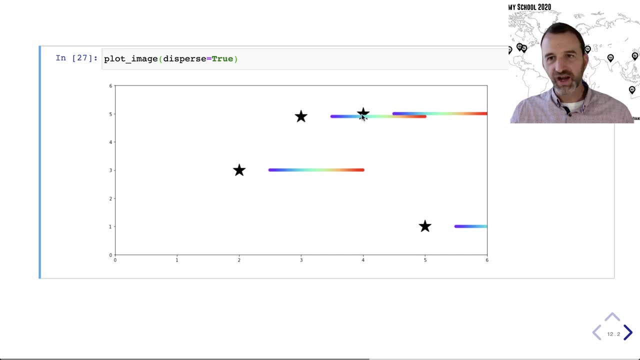 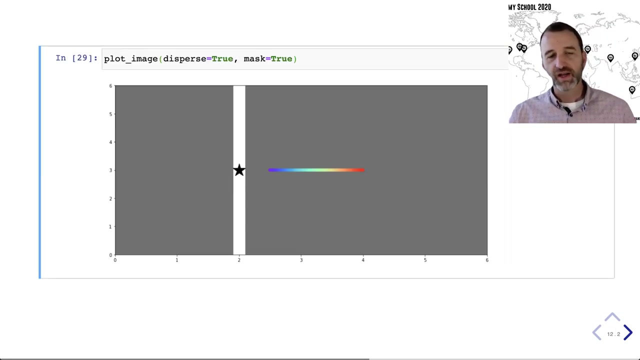 how do we know the light coming here? Is that from this star here? Is it from this star here Makes it a problem. So what we do next is we put in a mask. When you add a mask, you can block out all those other sources. 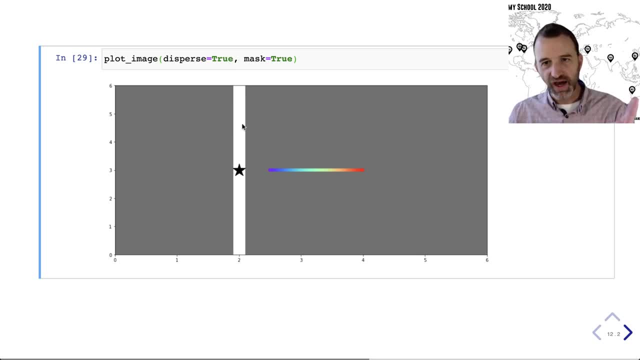 And you just have one source now or whatever is in this one line here. If I had another source here I'd get another spectrum. But you have a source In some allowed region And you have masks. that's blocking everything else. 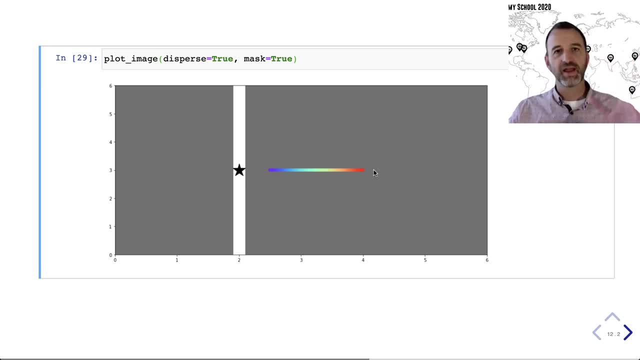 And so you get the light from that object coming through And it makes a spectrum because you have your dispersive element in A little bit of trickiness on the terminology here. So this mask that I'm using is very long And it's narrow. 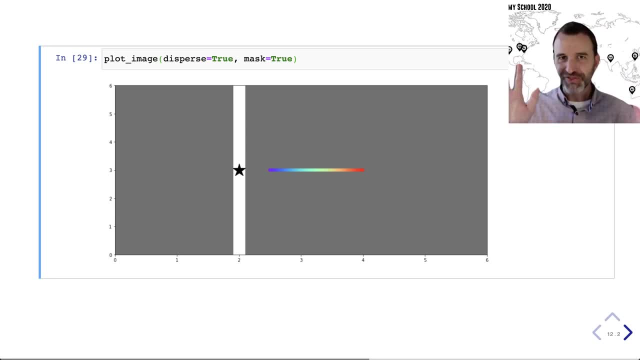 So we call it a slit, But this has nothing to do with the double slit experiment we were talking about earlier. This is not causing dispersion. Remember, before we put that mask in, this is not causing dispersion. We already had dispersion, It was already there. 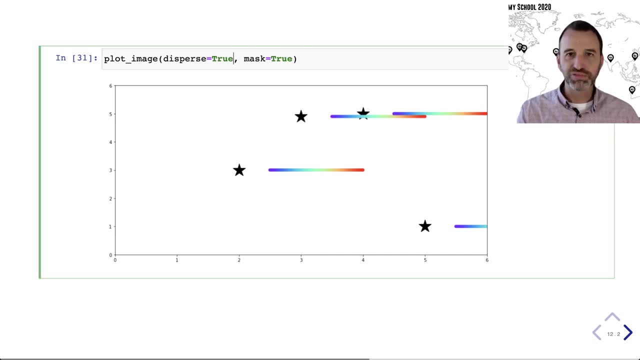 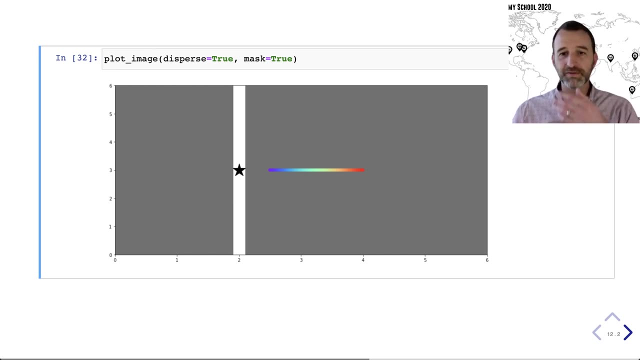 All we're doing when we're adding this mask is we're just blocking out light. It's just a. we call it a slit, but it's a slit mask, All right. So this allows us. now we can image this part of the spectrum here. 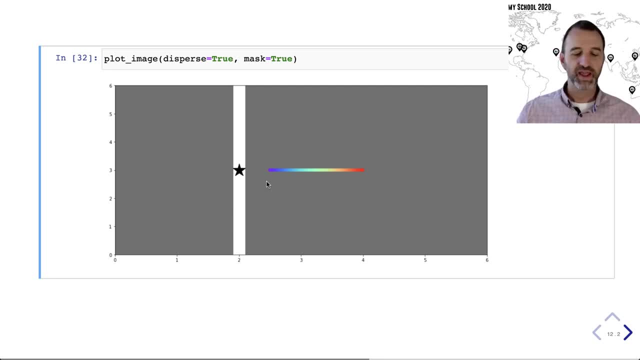 And we can record that data on our CCD And we can then analyze and figure out how bright is it at each one of these different wavelengths. One tricky thing that you should keep in mind is that your detector is going to be some finite size. 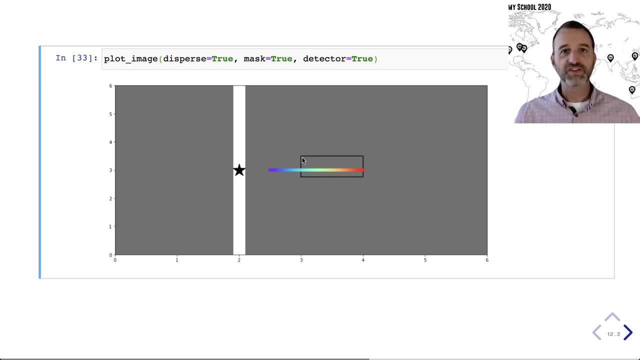 So maybe this little rectangle here is the size of your detector, your CCD. It could be smaller than that spectral trace that you have. So in general, you're only going to get some fraction of the electromagnetic spectrum on your detector And you may have some options. 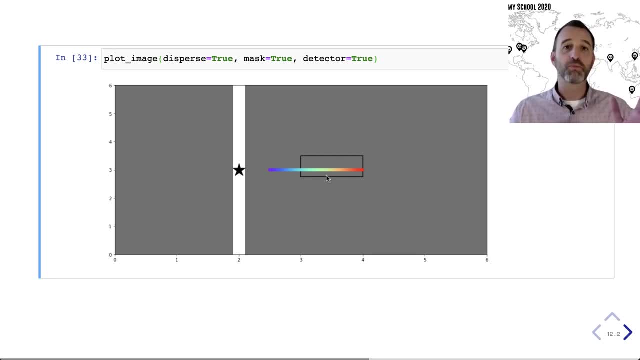 With your instrument to actually place this detector. or, more commonly, you can actually tilt the grating So you can make that spectrum move to wherever your CCD is. So you can image the part of the spectrum that you're most interested in. 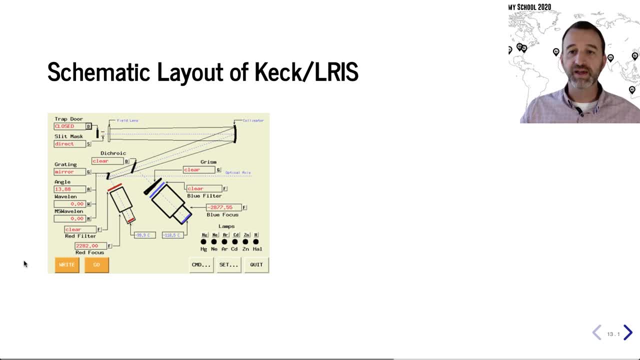 So let me show you a layout now. This is a real layout for the Keck LRES spectrograph. This is on the Keck 10-meter telescope, Keck 1.. So this is a little schematic here. It's just kind of giving you. 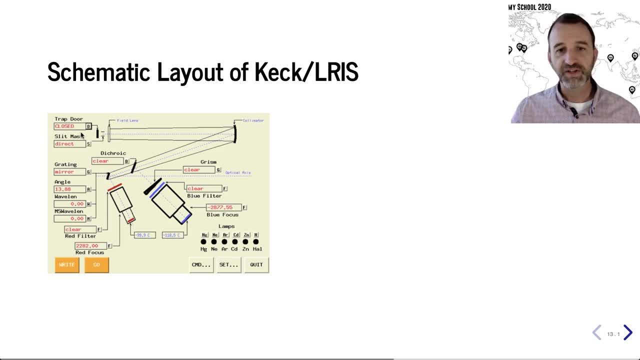 a cartoon view of how the instrument works. Light comes in through the telescope. It passes through that slit mask- just the mask. It goes through a collimator, And let's ignore this blue channel here. Some fancy spectrographs have two channels. 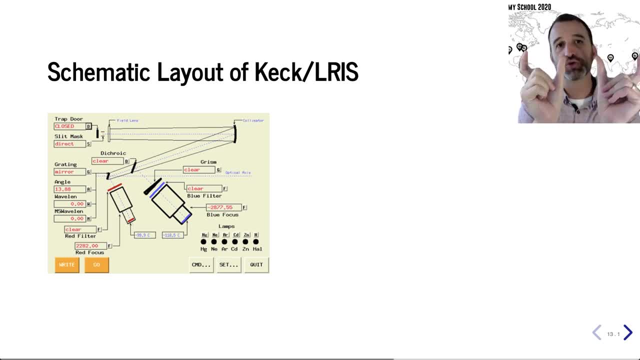 So you can have a detector that's imaging the red part and a detector imaging the blue part at one time. So if we just look at the light that comes through here, we can put a mirror here And the light will just go through and we'll get an image. 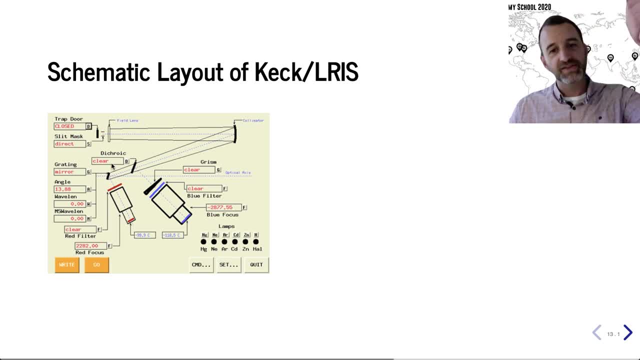 Or we can change this mirror out and put it in a grating, And then, instead of getting just a simple image we'll get, those spectra will start landing on our detector, which is down here, And we can change the angle of this so we can move those spectra across our detector. 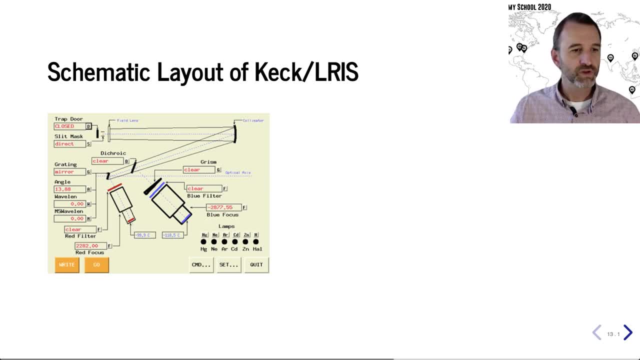 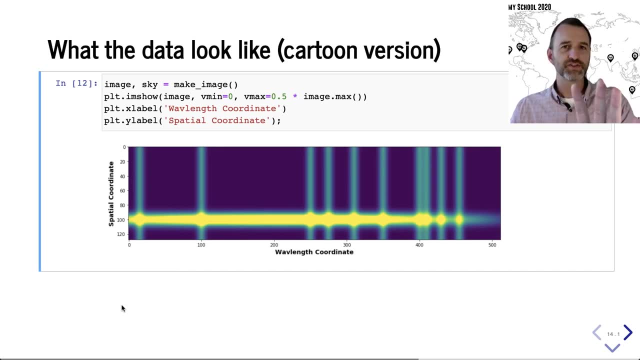 and get the part of the spectrum that we want. So, after we've done this, we've imaged it. what do we see on our detector? Well, we see something that looks roughly like this: This is a cartoon. This is not reality. 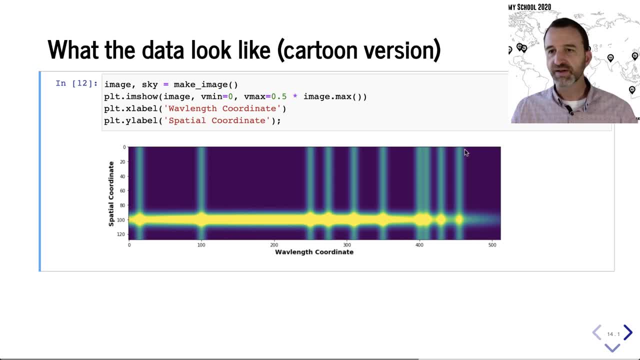 But this is demonstrating what you're going to see. So we have our CCD area here And on that we have a light From a target. that light is dispersed across this way, So it's important to understand that we have a wavelength coordinate. 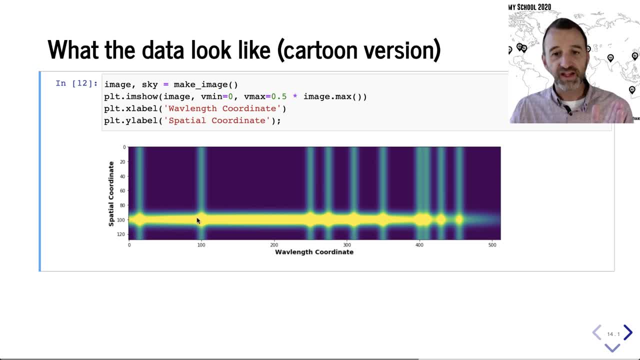 So as we move from left to right here, we're changing the wavelength that we're looking at. Each one of these is a different wavelength bin. moving left to right, As we move from top to bottom, we're changing the spatial coordinate. So we have an object which is located around pixel 100. 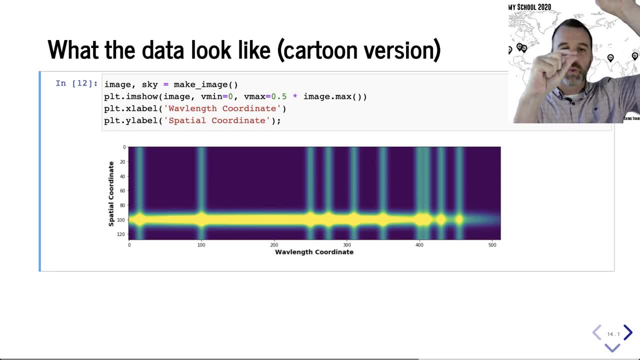 So we have that long slit in some spot. in there We're getting light from a source And there's no source at any other position. It's there. So if we had another object over at position 40, we'd get another trace across the field like that. 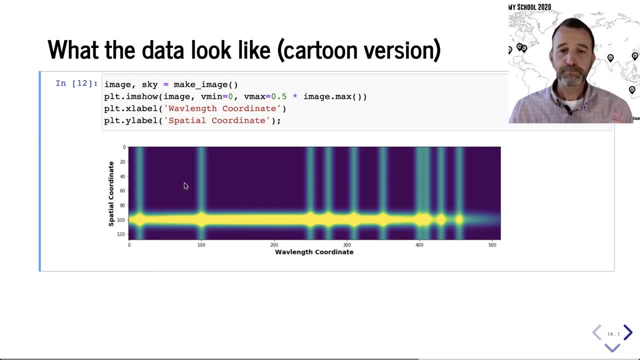 But for this example, we only have one object in our slit, our mask. Now, you may be noticing, there's some lines that extend across the CCD at certain wavelengths, At this wavelength, for example, at wavelength 100, whatever units those are- we get light. 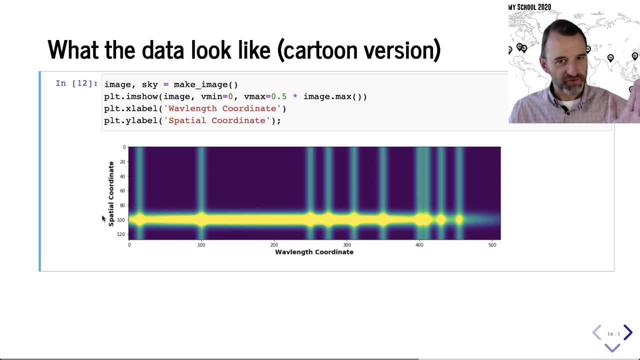 at any position we look at. Keep that in mind. This is spatial position. So at any position you look at, at certain wavelengths, you're getting the same amount of light. So what this is telling you, this is our background. So this could be light from just the air around us. 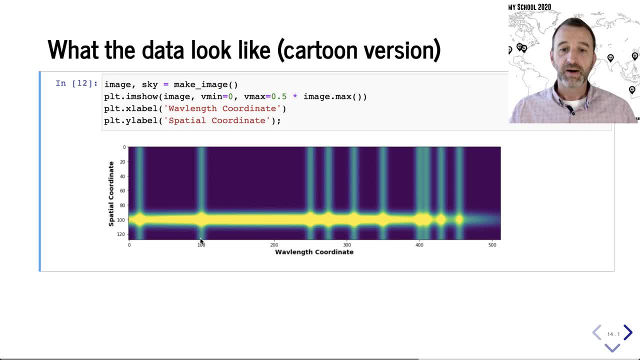 The spectrograph is picking that up- the air and the atmosphere. So no matter where you look, you still are looking through air, So you're going to get some amount of light shining through And that air above you does have some continuum. 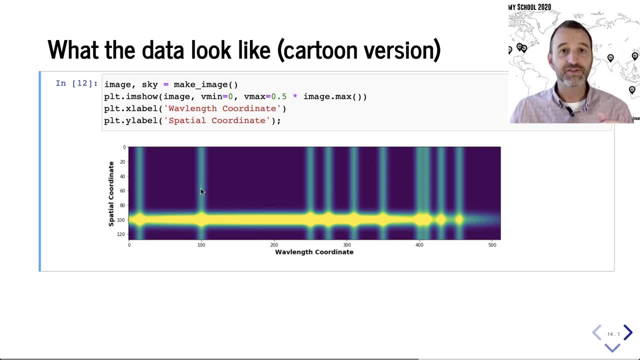 But most importantly, it has some emission lines. So the night sky It's a gas, It's excited, It's at some temperature, So it is going through transitions and producing emission lines, just like gas in a laboratory. So these are very important. 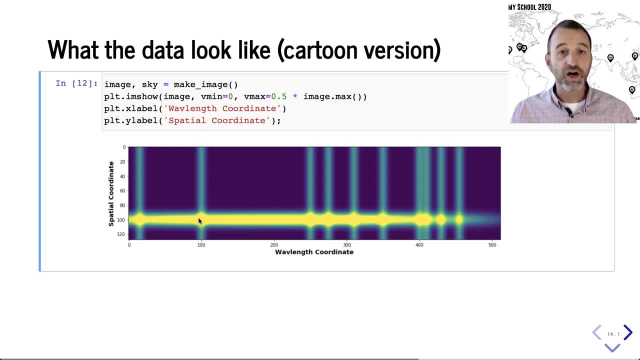 They can cause a background, a wavelength-dependent background, for your source. But they have some advantages. We can actually use these for wavelength calibration. I'll just note that if you had real data. so I'm doing this in cartoon version, So the lines are going straight across. 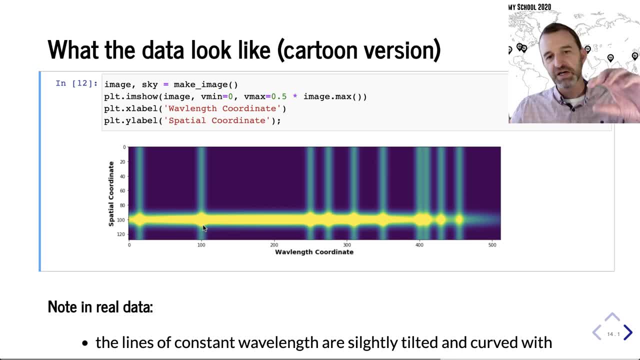 So I'm doing this in cartoon version. So I'm doing this in cartoon version. So I'm doing this in cartoon version, And the wavelengths are straight up and down Real data. the trace is going to be kind of tilted on your detector. 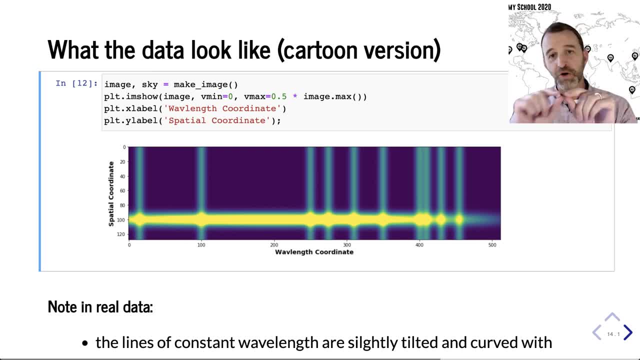 And these wavelength lines are going to have some curvature in it. So figuring out where each one of those wavelength bins is, as a function of position on your detector, is one of the tricky parts- one of the most tricky parts actually- of reducing a spectrum. 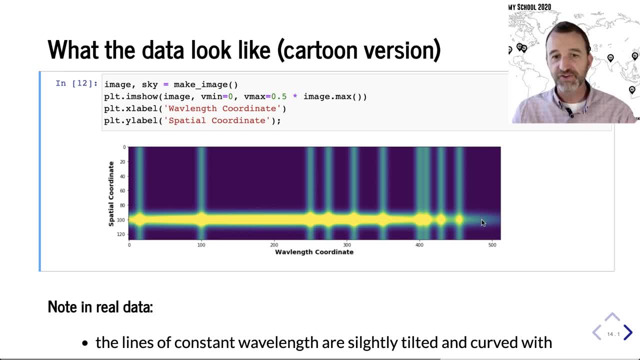 So what we want now is we want the light from this trace object here as a function of wavelength. We want to know what the flux density is at each one of these wavelengths. We want to know what the flux density is at each one of these wavelengths. 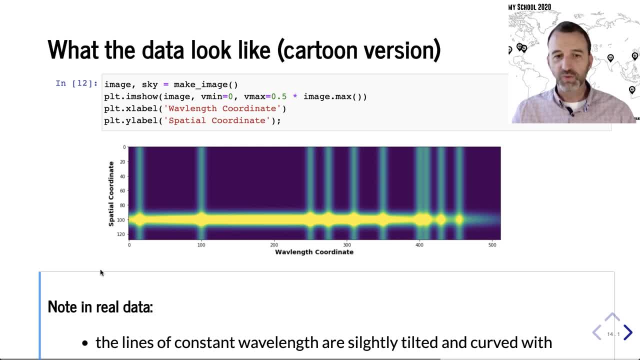 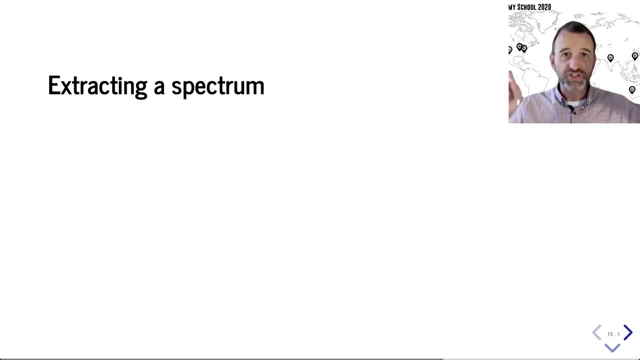 Here we have 512 in this example. So each one of those, how bright is it? And this is called extracting the spectrum. So we take that two-dimensional data and we're going to get a one-dimensional answer which is just the flux density as a function of wavelength. 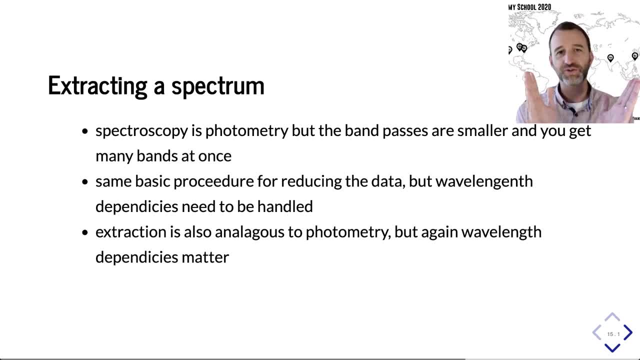 So I've kind of said this before. Just remember, all we're doing here is we're doing photometry, but we're just doing it many, many, many, many, many times at once. So for each one of those wavelength bins we have light. 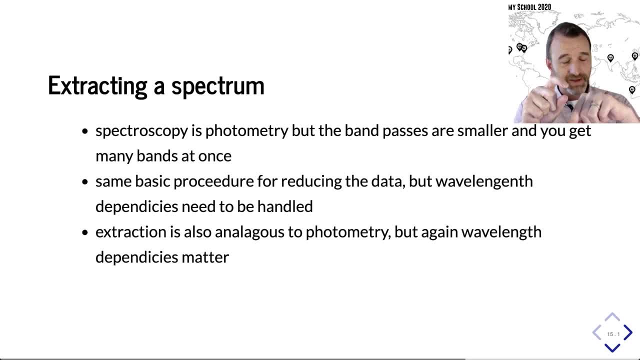 from our source and we have background light And what we need to do is we need to figure out how much light are we getting from our source and how much is contributed by the background. remove that background component and then we'll have how much is coming from our source. 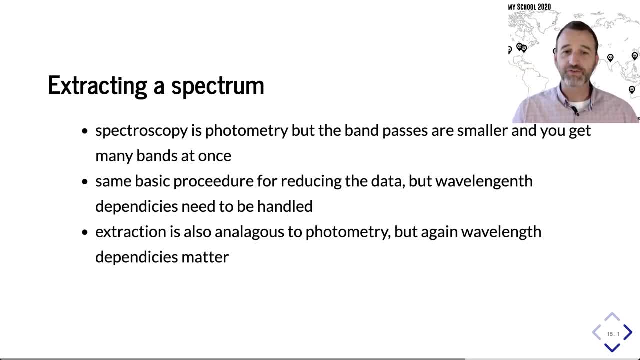 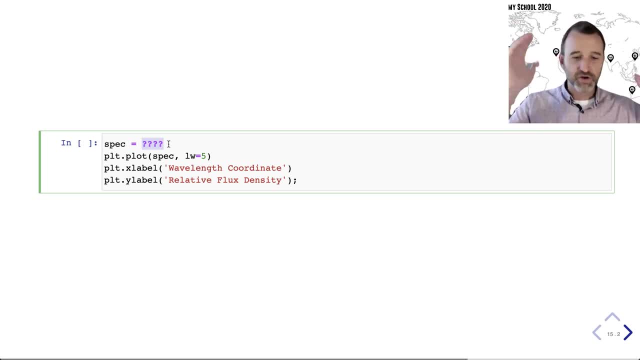 And we do that for each one of our wavelength bins. We got ourselves a 1D spectrum. So first thing let's do is let's extract the spectrum, Let's take the whole image and just for each one of those columns we can say: well, this is a one wavelength. 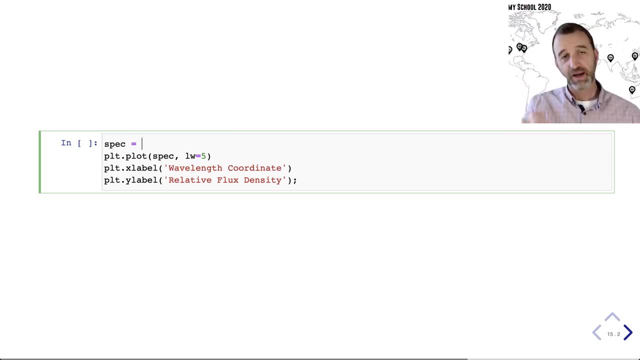 So let's just integrate along that entire column and we'll get the total amount of flux on the image. So to do this here, we just take the image that we've generated and we're just going to sum it along columns, which is axis 0.. 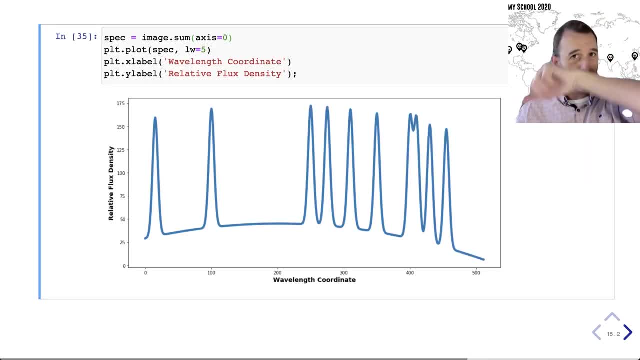 There we go. So this is the whole image now, the whole 2D image that we have just integrated. we've marginalized, if you want, over one axis, And then we're going to take the wavelength coordinates. We have those 512 measurements that we've got now. 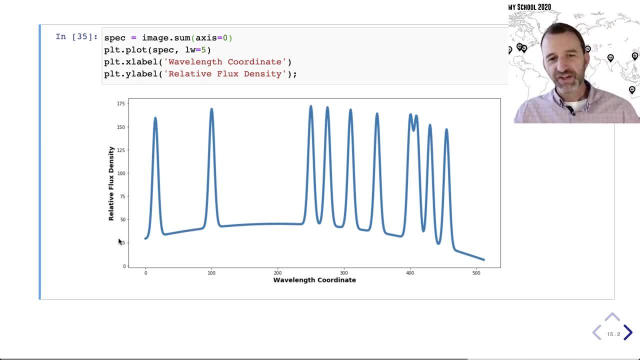 And at each one of these wavelengths we have some amount of total light on the image. So you can see there is this kind of curve here. That's our trace, that we want, But on top of that there's all these emission lines. 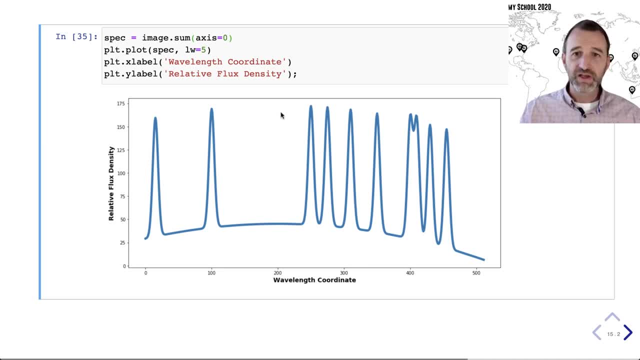 from the sky And of course we have to deal with this. So one thing we can do right off the bat is we can narrow that aperture for extracting our source. We can just kind of put it where we know the light comes from our source, because it's not everywhere. 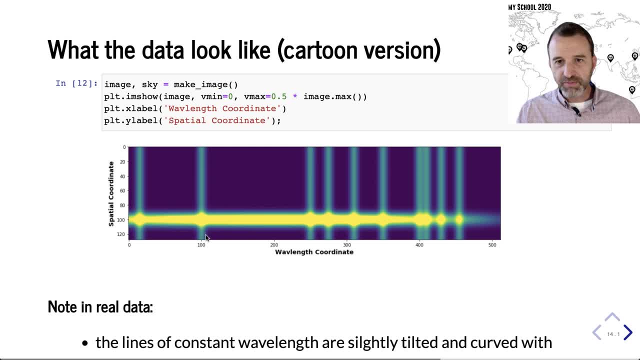 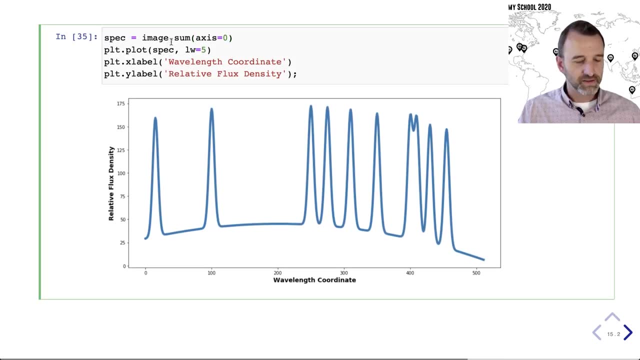 So what we just did is we integrated all the way from top to bottom on this image for each wavelength, But our source is only here. So maybe if we just extract this region here- maybe from pixel 80 to 120, then we can get just light. 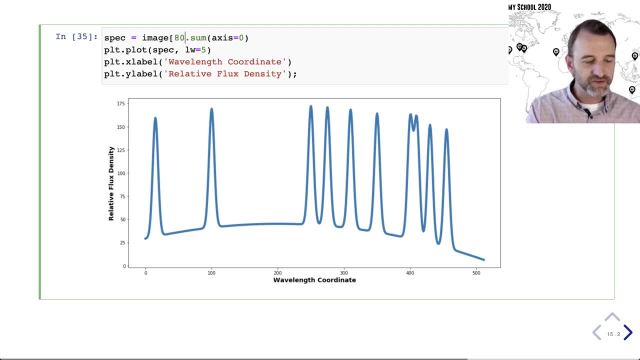 We'll be more dominated by light from our source. So we'll just do columns 80 to 120.. We'll do the same process And there we go. So we still have light from the background, but now we're a little bit. 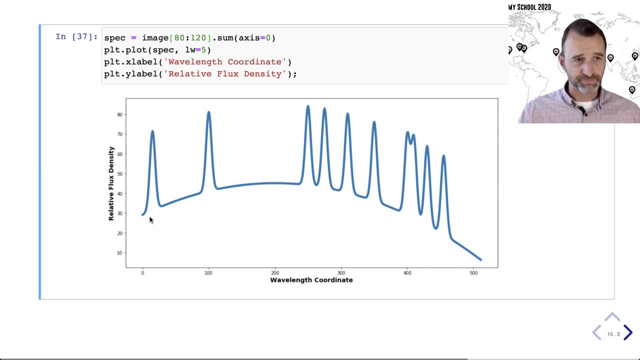 a little bit more weighted towards the target light that we care about. So then, the next thing we need to do is, of course, we need to subtract off the contribution of the sky as a function of wavelength. So what we do for this is: we have our sky measurements, which 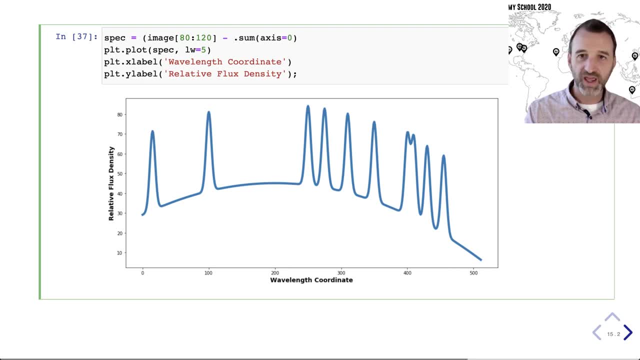 could just be the. we can just use the image. So we'll take the image data we have And then in a different part where we don't have that trace, we'll just say, OK, How bright is the object here? 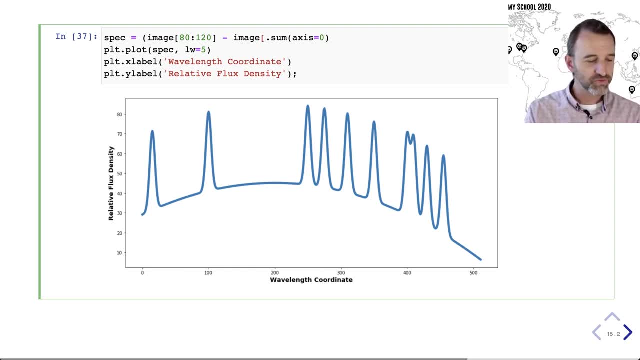 So that's we need to. so we have 40 columns here, So we're going to go from, maybe, column 20 to 60, where we have no light, Sorry, row, row 20 to 60. And then we just take the image where we have the target and the image. 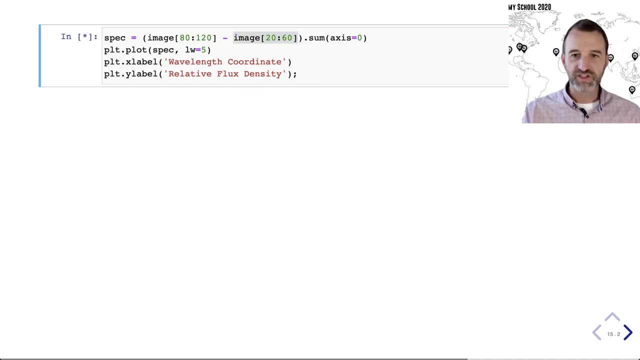 where we have the background. subtract off the background and we'll have just light from our target. So this is very analogous to what you do for photometry: You always have to subtract the background light, But now we're just doing this 512 times. 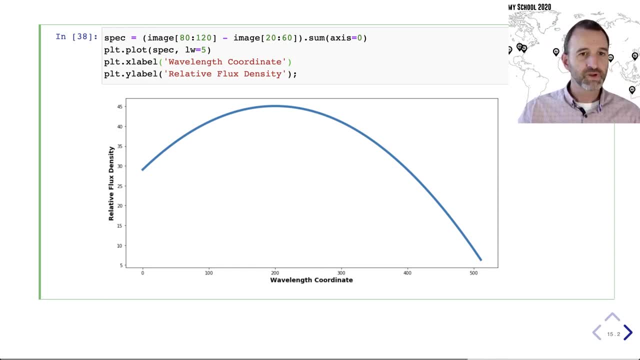 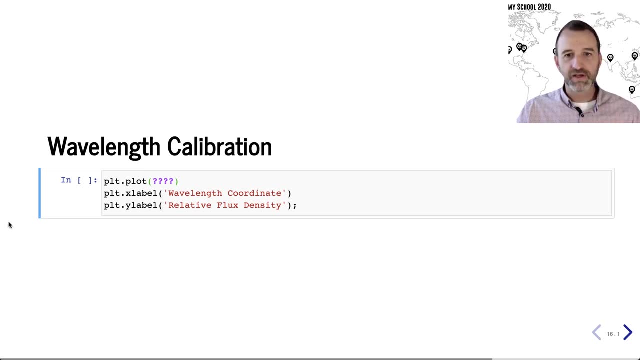 At once. So now we have some wavelength coordinate here, but we don't know what those wavelengths are, So we need to calibrate this as well, And the way we can calibrate our wavelengths is by using known emission lines. So a popular way to do this is to take a lamp where someone 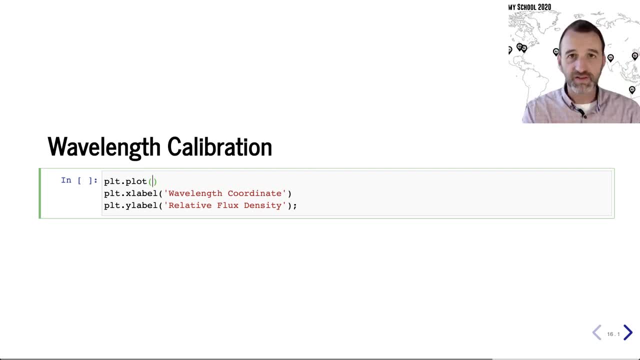 has taken the time in the laboratory to calibrate what each one of the wavelengths are that are emitted by the lamp. We can just use skylines maybe in this case. So if we use just our sky background, we can just use that. 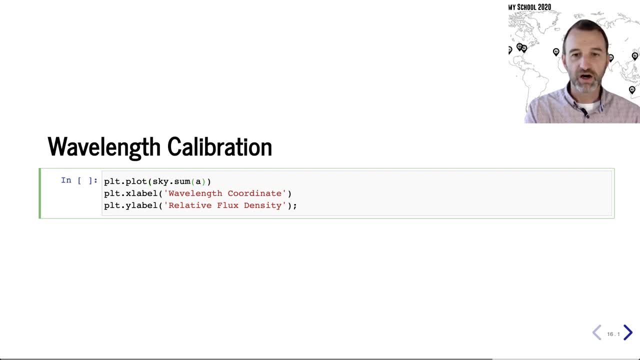 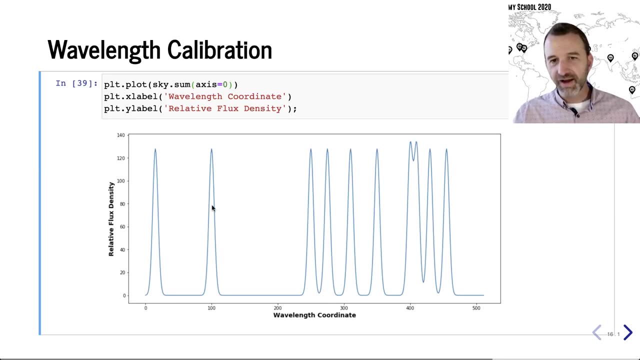 OK, And we'll just sum that over columns: we get this. So now, if I know that this line here- maybe this is an oxygen line, it has a wavelength of 55, 77. I know this line, I'm sure it's this. 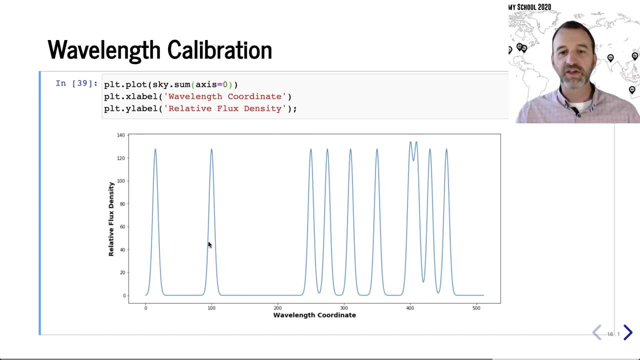 I can identify these other lines. These are OH lines or some other lines. Now I can do a mapping between the known wavelength of this line and the coordinate here and I can create a wavelength solution. So then, if you give me any wavelength coordinate, 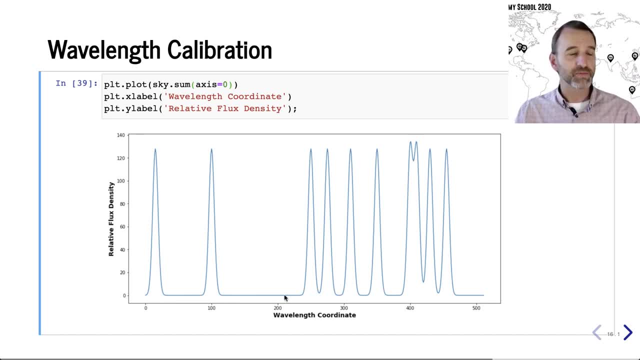 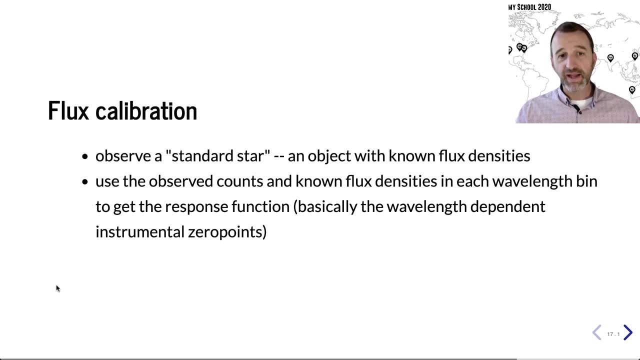 I can say: well, this is the wavelength, This is the corresponding wavelength in Engstrom's. You also may want to calibrate the flux densities. So each one of those wavelength things you're getting counts at this point. So we know that we have 10 counts in this bin. 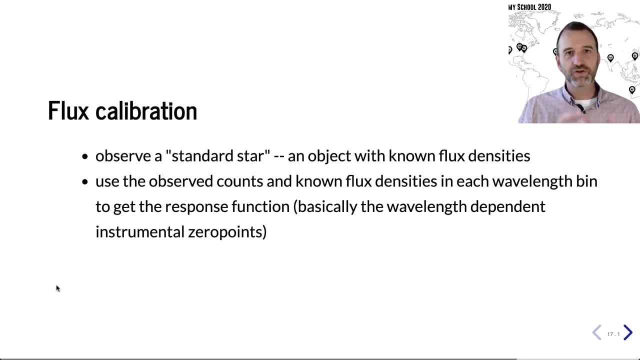 But what is that in flux density? So the way we do this is the same way we do it for photometry. You observe a star that has a brightness that's already been calibrated, So we know, in that wavelength bin, the brightness of those. 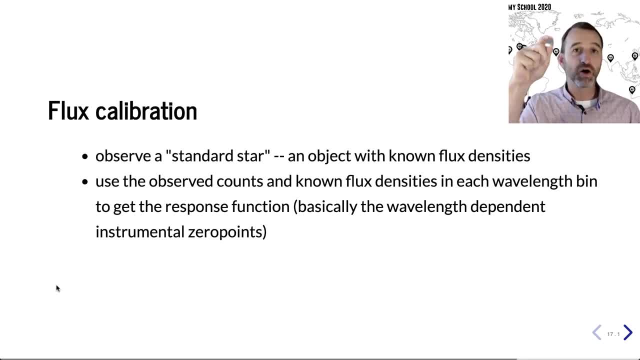 of this standard star. It's been calibrated And so we say, OK, well, we got 100 counts in this bin and it has a flux density of this, So then we can calculate effectively a zero point for that wavelength bin. 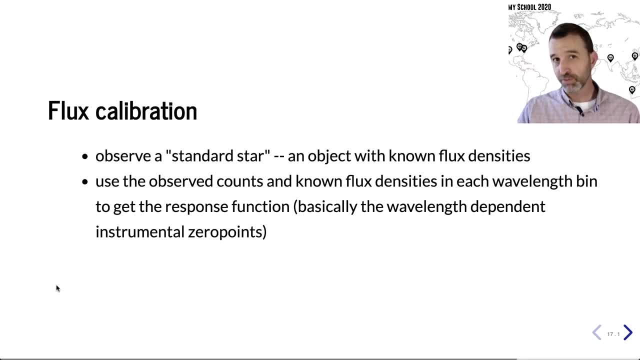 And we can do this for every wavelength bin. Each wavelength bin is going to have a different zero point in, using kind of a photometry speaker, And so we can calculate, as a function of wavelength, what our zero point is, and that will give us. 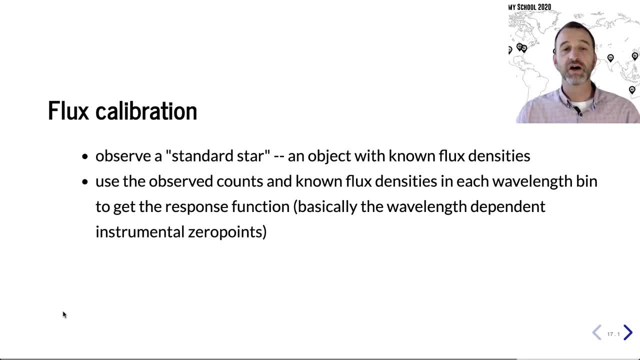 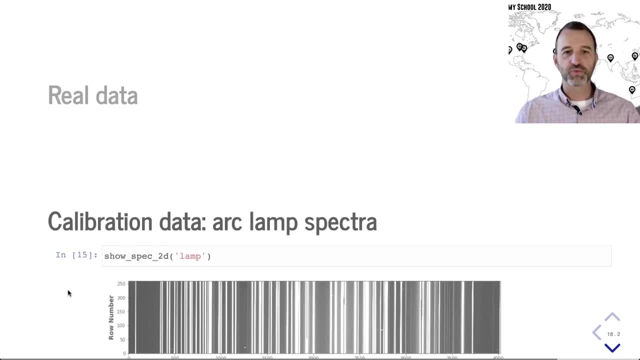 a way to take that whole spectrum we get and turn it into from counts to flux, the flux density. All right, so I give you kind of a cartoon version here. I want to show you some real data now. This is a real spectrum of an arc lamp. 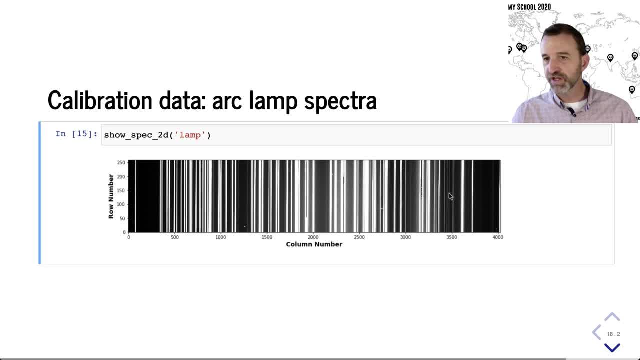 So we have column number here, row number here. Dispersion is happening along this way. So all these lines here, these are lines of constant wavelength from a lamp that was illuminating the slit, And we know these wavelengths. People have calibrated these in a laboratory. 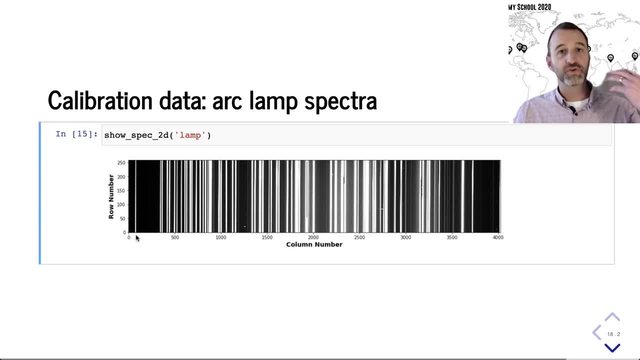 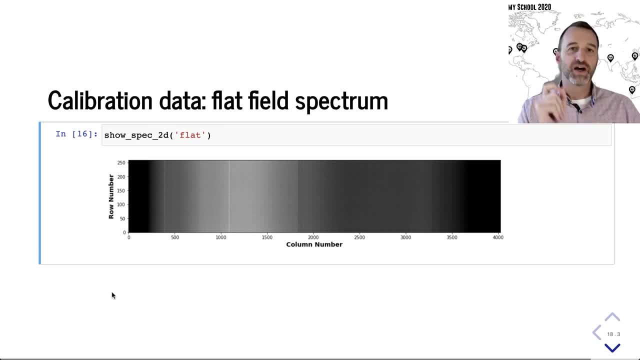 So we can convert now from pixel coordinate and column number into wavelength number. Next thing we can do is we might want to flat field our data. So you remember, in each wavelength bin we have a whole set of pixels And there might be differences in the quantum efficiency. 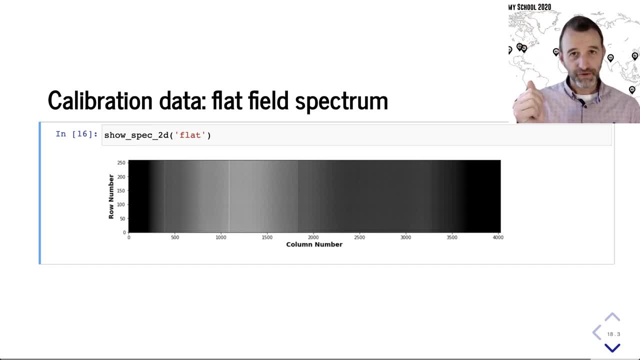 of the detector from pixel to pixel. So we might want to correct for those Now to do this. when you're doing imaging you may be used to taking one image where you assume all at the top of the aperture you get the same number of photons. 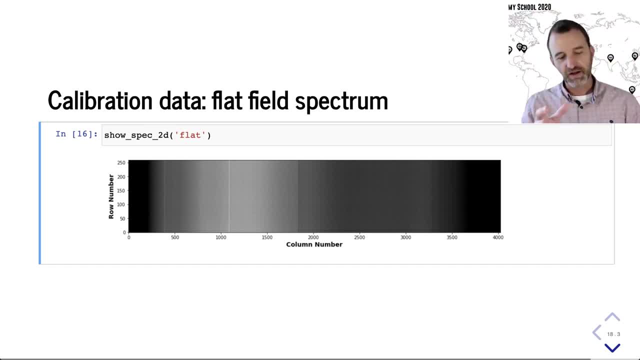 that you had in the first incident And they go through the whole optics on the detector. You can just say: well, this pixel got 10,000 counts and this one got 9,000 counts. That means well the ratio of this. 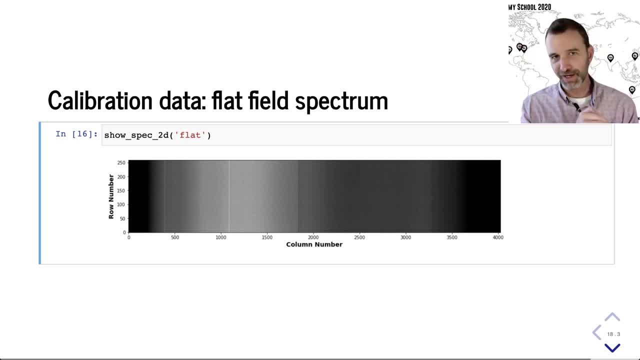 is telling me something about the relative efficiencies of these two. It's a little more complicated with spectroscopy. I can't just do that for this whole image here, because the brightness as a function of column here has something to do with the spectrum that we're illuminating the detector with. 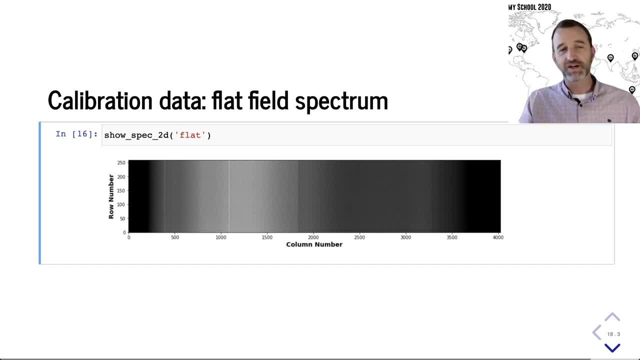 So we may have some lamp that might have more red photons and more blue photons and red photons. You don't know the temperature. We don't have the calibration for those things in exact terms. So what we do is we say: OK, we know now. 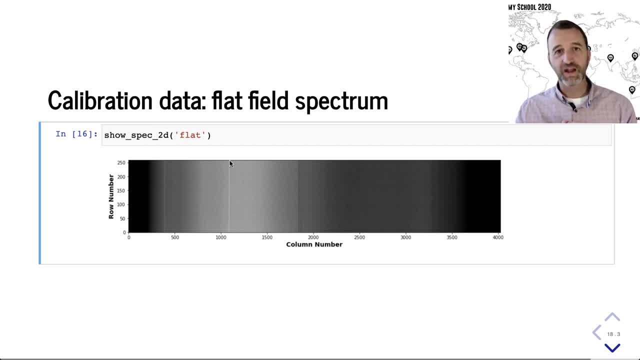 from our wavelength calibration that here is a line of constant wavelength And so along this line we're going to say what is the typical number of counts? Maybe it's 5,000.. So say OK for each one of these pixels in that wavelength. 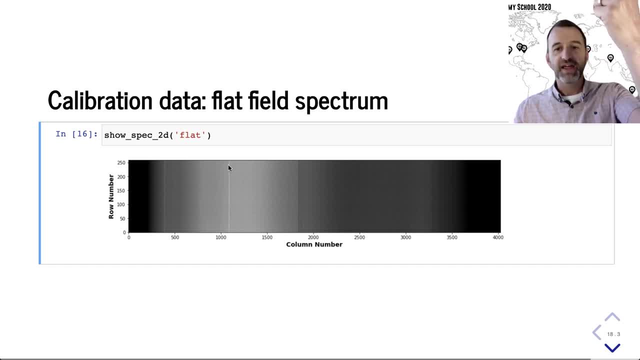 bin. we're going to divide those by 5,000.. And then we'll get the relative sensitivity from pixel to pixel. So we can use that to calibrate our images to correct for field variations. Then we can take a standard star observation. 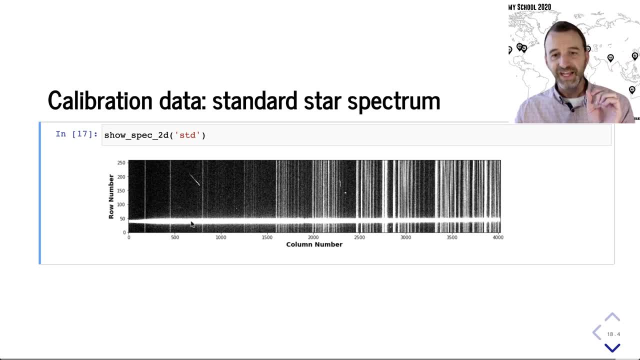 So we'll go to again a star. We know the flux density at each one of these wavelength bins. We measure how many counts we get And then we can get our conversion factor. We get a function to convert from counts to wavelength. 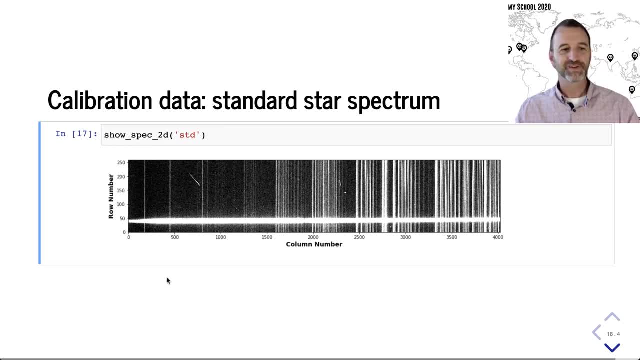 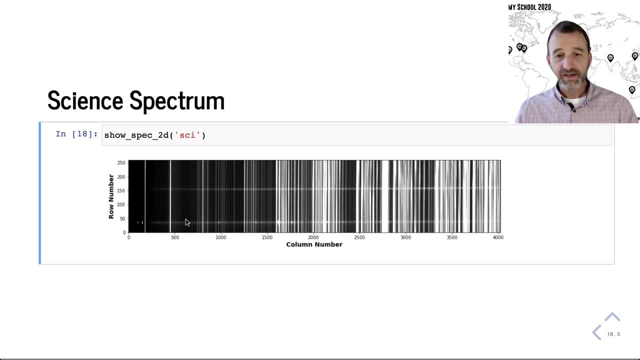 Sorry, counts to flux density as a function of wavelength, And then, finally, we can move on to our science spectrum. So this is a real science spectrum taken by Keck. This is the object that we're caring about here, And then when we do the hands-on session, this is the object. 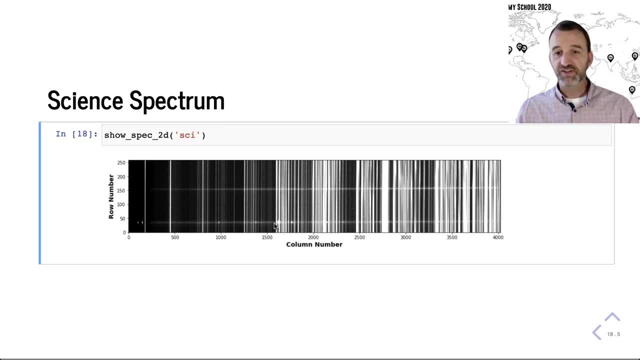 This is the data you're going to be working with. So this trace here is actually of a galaxy. You can see it's got little emission lines here And so if we can extract this spectrum and we can figure out the wavelengths of these emission,